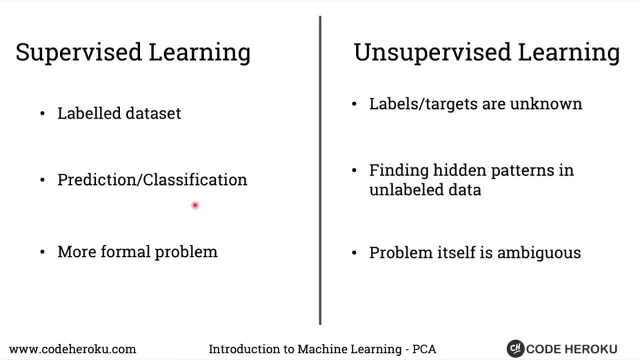 predict something or you're trying to classify something, whereas in unsupervised machine learning algorithms. we just said that it is important in some cases to find hidden structures or patterns in the data which might not be obvious and, in a general, at a very high level, we said that it is more of a it's. 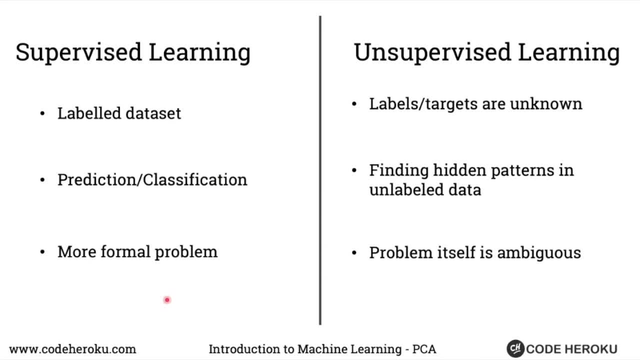 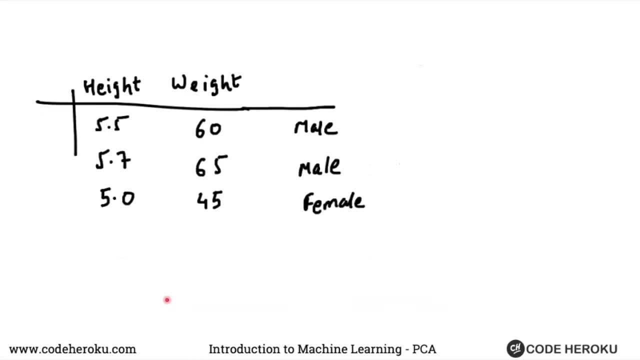 more formal problem than unsupervised machine learning, because when you're doing unsupervised learning your end goal sometimes is not known. you don't know things that you don't know right. let's say you're given this data set. this data set has two features over here: the height and the weight, and based on 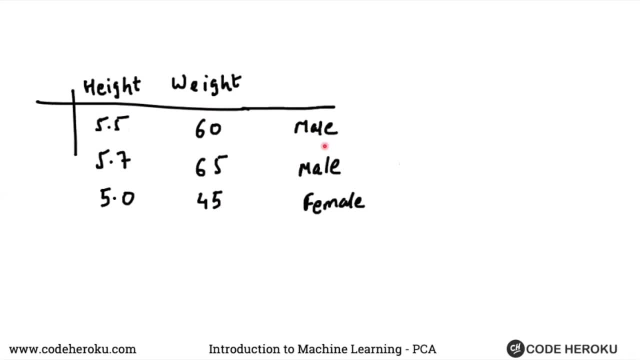 the height and the weight, we are trying to classify whether this person is either a male or they are a female. so we are given only three examples over here. okay, so, with looking at these three examples, you- even though it's a dummy example, let's say this was given to us and our 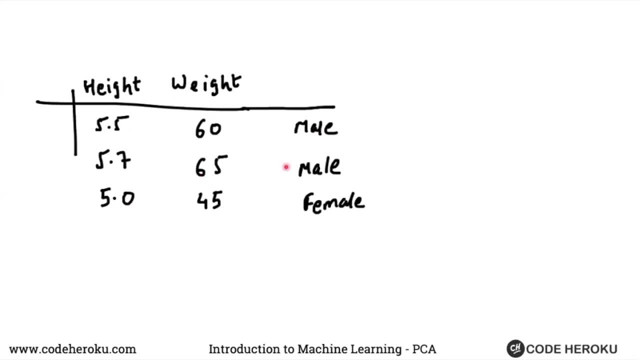 job is to make a classifier which can learn to predict based on, or to classify based on, the height and the weight. you want to say whether that person is a male or a female. so let's say you plot it on a 2d graph like this: the males. 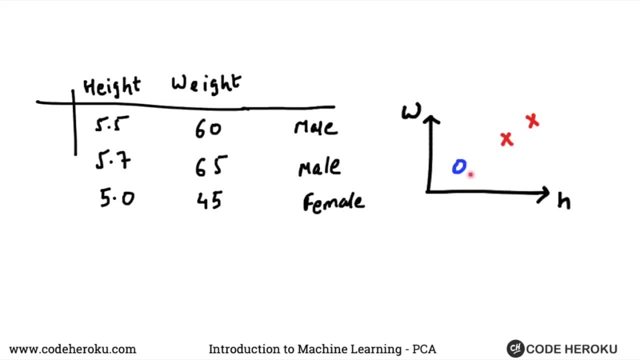 seem to fall in this region of the graph and the females are somewhere over here and we run this curve over here. similar order for each of these symbols. so you end up creating a classifier which might come up with a solution like this one, and we have already seen several techniques to create a. 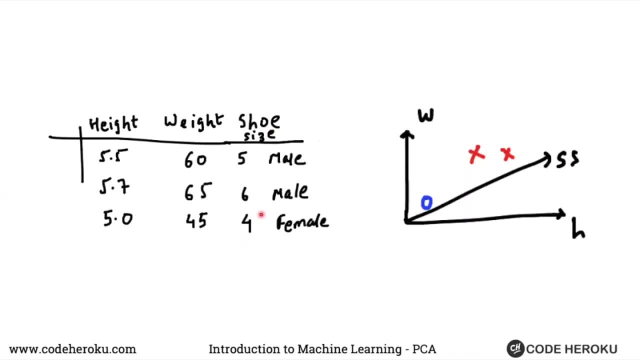 classification boundary like this one. so now, let's say, I add another feature over here which is called shoe size right and this shoe size, and you can imagine that this shoe size is somehow correlated to this sobre un town, wes height and weightasse. toe size right. 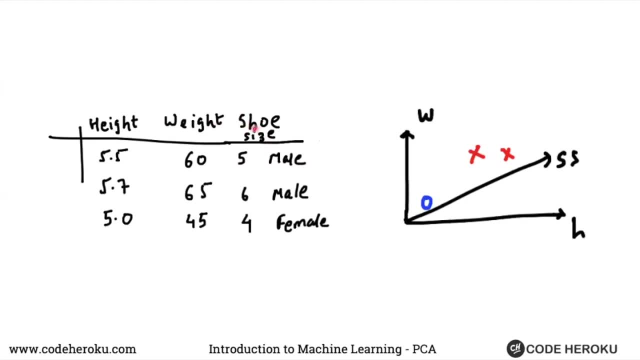 is over here is gone, right. So as much you can imagine, this is something that what is top stop at the end of this channel classifier Right. So people with no higher, with the bigger height or know who are taller, they might end up having a larger shoe size. 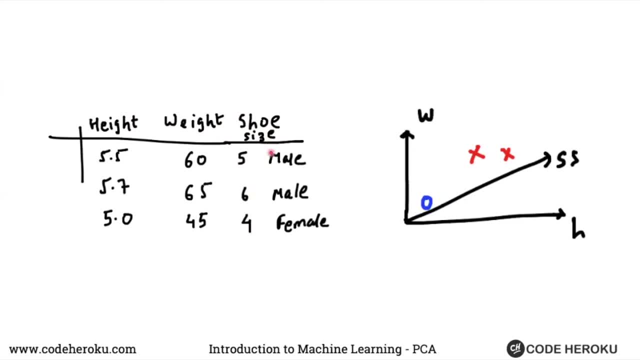 But we still choose to use it And we think that, no, adding more features to our data set might help. We don't know yet. OK, but we just added one more feature over here saying we'll use shoe size as well. So what's what happens now? So our 2D graph now turns into a three dimensional plot. 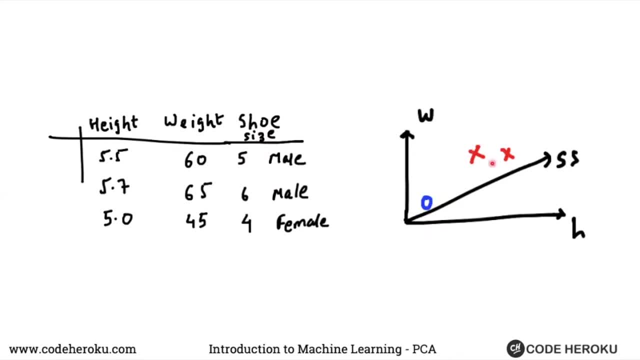 And We added those know our readings again. Now I want you to observe and tell me some differences that you see between these points in a 2D plot like this one and a 3D plot like this one. We just added one more feature over there. 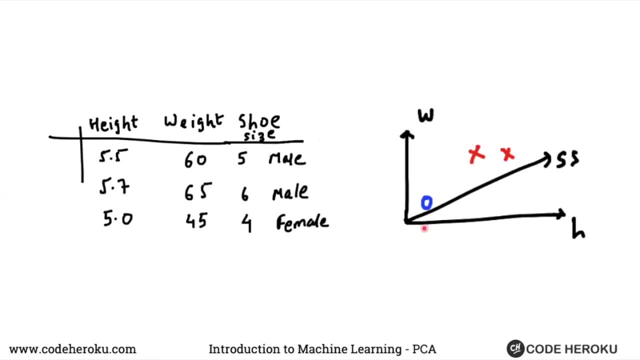 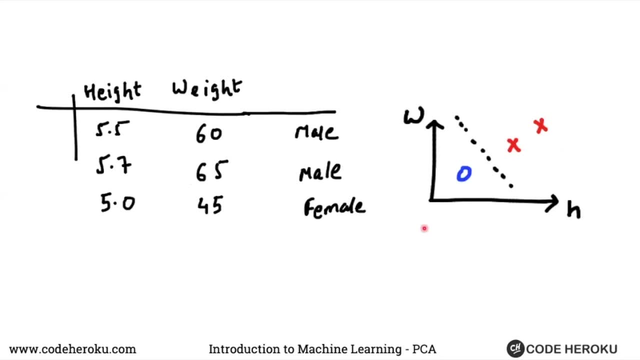 And I want you to see. I want you guys to tell me What are some of the differences that you see in versus having the same data set plotted in 2D. And now we added one more dimension, So there is another dimension with a shoe size. 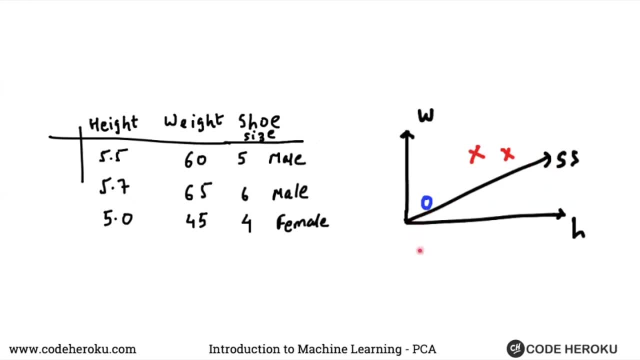 Which is going, you could imagine it is going outwards, and you have these points over here now. So how are they different? How are these two plots different? Can you tell me What are some of the differences that you see, besides the fact that there is a third dimension? 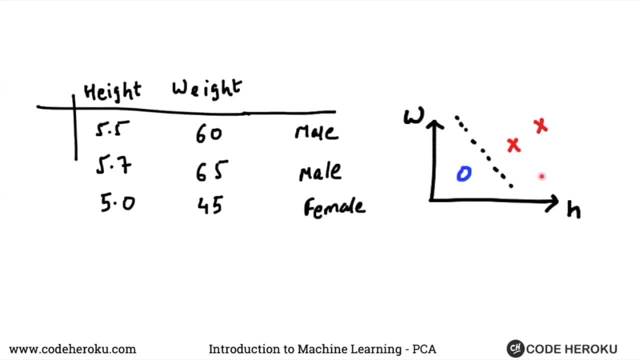 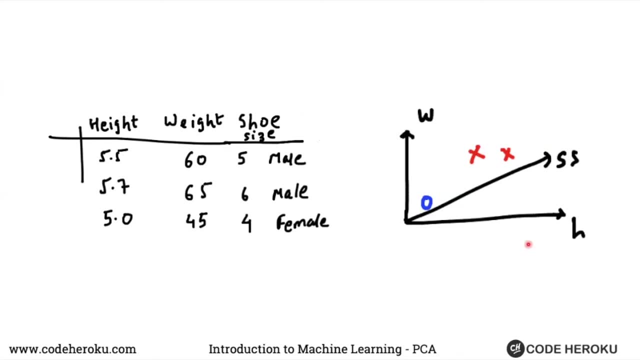 Over here. if you observe the entire, this entire points seem to be much closer together compared to this one. As soon as we added a third dimension over there, your points in the space are more spread out. Am I correct? Let's say: what does our classifier do now? 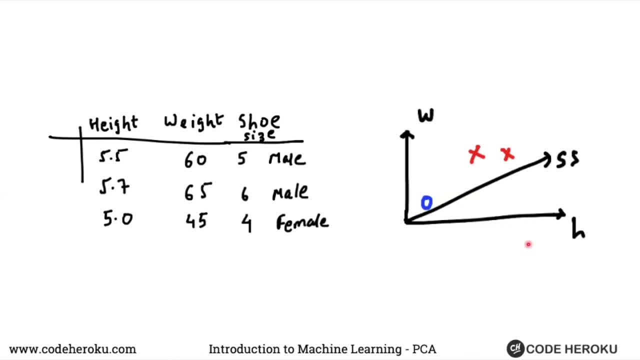 A classifier sees A pattern like this, And what it might end up doing is create a decision boundary which might look something like this one. So it thinks that all the X's Necessarily need in this space over here, And all the zeros, or all the females, are somewhere in this region. 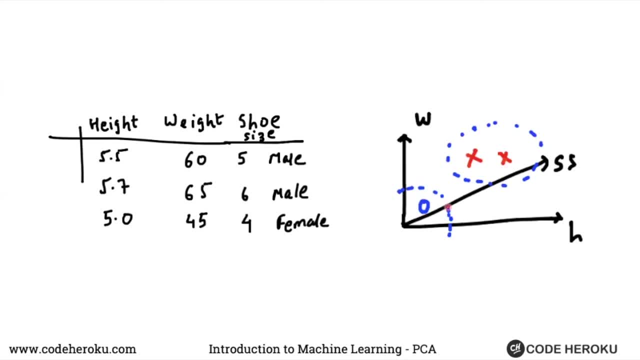 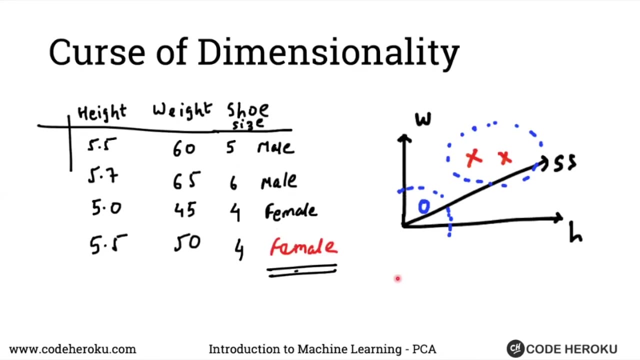 Because it thinks that, because it has seen only three examples, Right. What it says is: I think all the zeros, I think all the zeros must fall over here in this, this region. So what happens if someone gives us a new row to classify? 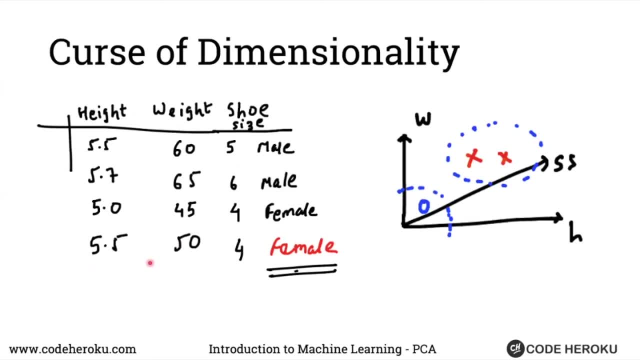 So over here someone gave us a new row to classify And we said They were. They told us that the height was 5.5.. Weight was 50. And the shoe size is four. And because now we had a four over here as well. 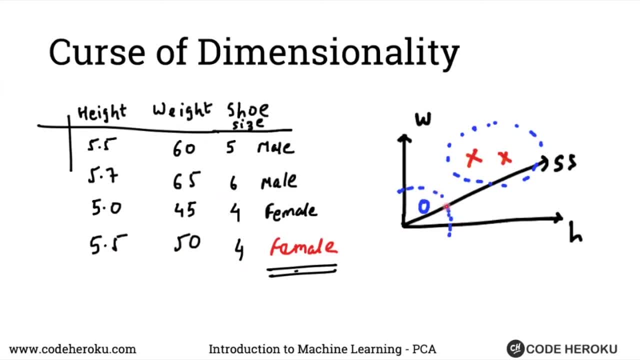 And our classifier thinks that everything that in this region which is close to four Must be a female. We predicted female. Is it necessary that In every instance, If the shoe size is around four, Should you classify that person as a female? 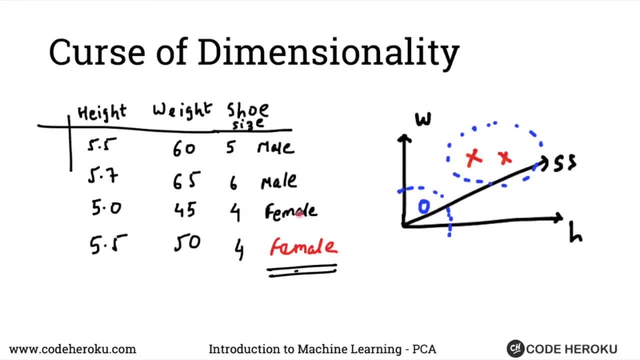 Or do you think it was just one instance when this has occurred And we shouldn't generalize that And we shouldn't learn too much from this Exactly? There are other features that matter as well, But what is happening is Because we have very less examples over here. 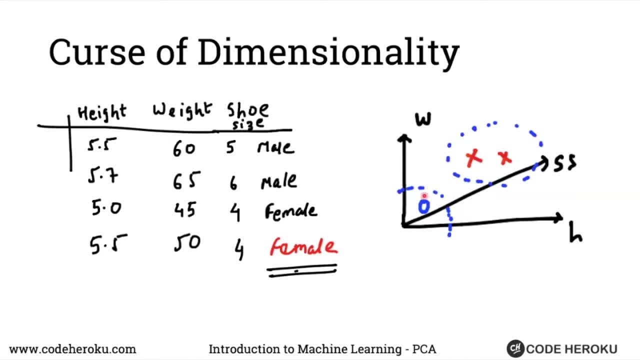 And more dimensions. Our classifier is In technical terms. We are overfitting our classifier over here Just by looking at few examples, Because the number of dimensions are more. What we think is Everything that looks like this Must fall in this region. 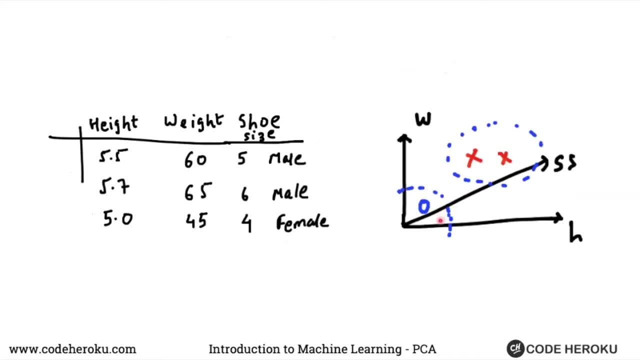 Adding another dimension is not necessarily a good idea And, conversely, What we could also say that If you are given lot of dimensions, Not necessarily all dimensions should be taken into account, And this is what we call sometimes as curse of dimensionality. 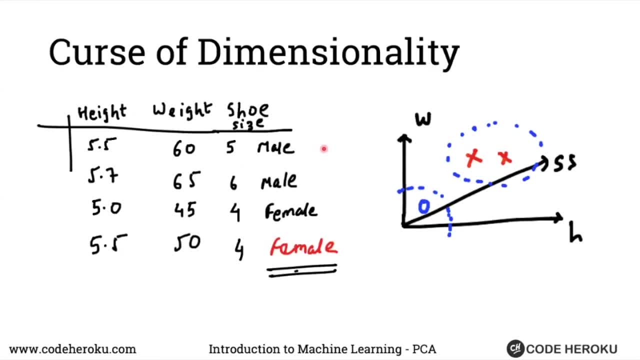 What ends up happening is, As you go on, increase the number of dimension. One: Your data points get more sparse in this space. They become increasingly away. What that does is One: It increases the size of your search For your classifier. 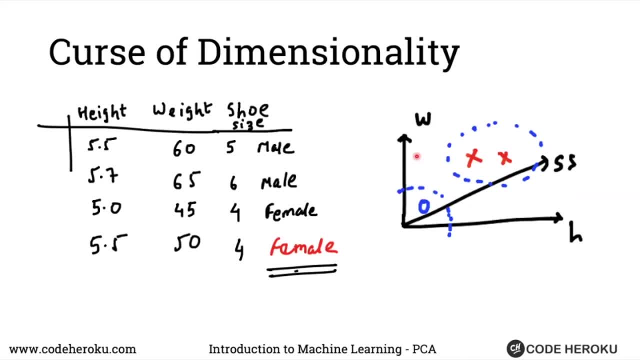 The time to train your classifier will be much greater, Because you will have to search through a bigger space Than you would have to do with fewer dimensions And two. What it also does is It over fits your model. What we do is: 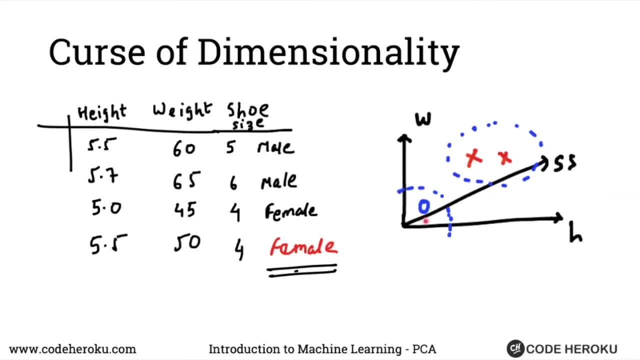 It turns out that When you add more dimensions, You try to become overconfident. You think that Because this point lies specifically in this region of the space, It must be that All such points Are what constitute A female. 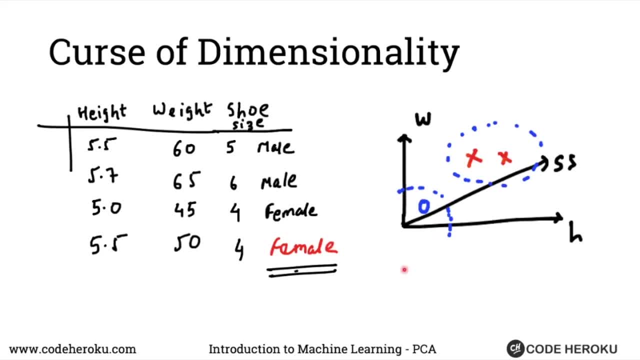 Example. So that's what we are trying to get To today. What we are trying to see is: How can we reduce this dimensions In a meaningful way Says that we don't lose information that we have, But yet we are able to get better results down the line. 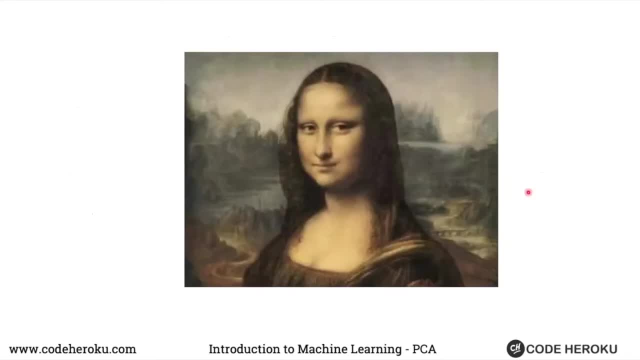 So I have a task for you today, And this will give you some insights on How we are going to go about reducing the dimensionality. I want you guys to Draw this painting Which you see in front of you, And I know that you won't. 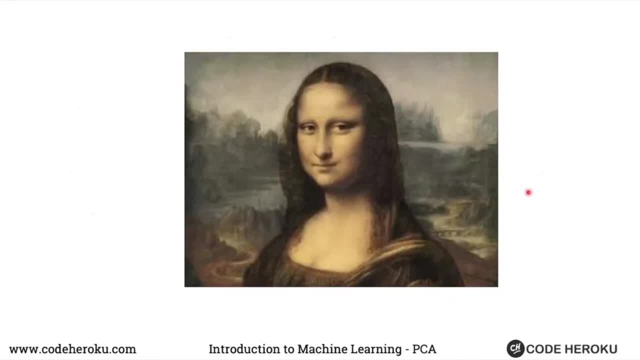 Excel at that, Right, But try to do As good as you can. Okay, Get your creative hats on. In next 30 seconds, Draw the best version of Mona Lisa As you could On paper. Trust me, I'll tell you how that relates to. 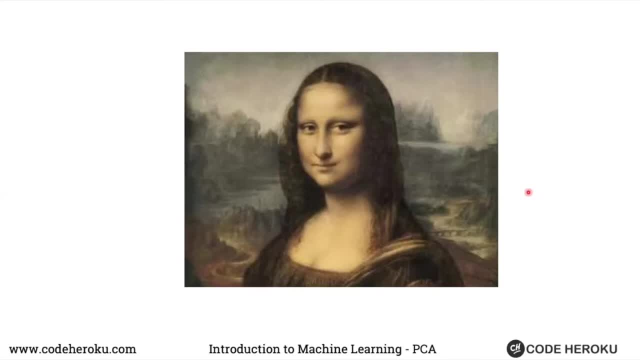 Dimensionality reduction. So What we are going to do Is We are going to Draw The best version of Mona Lisa, Which is Dimensionality reduction, All right. So if you are someone like me Who is not really artistic, 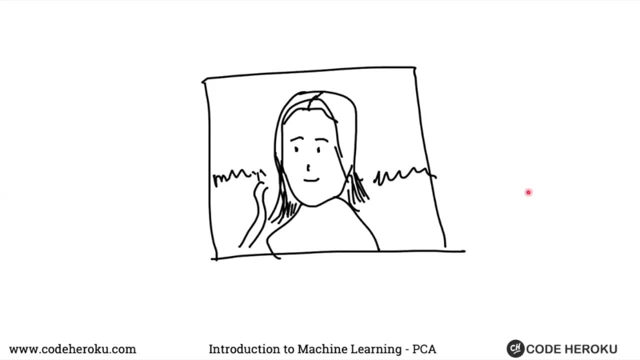 You would end up With something like this: And if someone Has a Better picture than me, Kudos to you, But if you drew Even worse than this, Then you should go And get some drawing classes. Okay, But 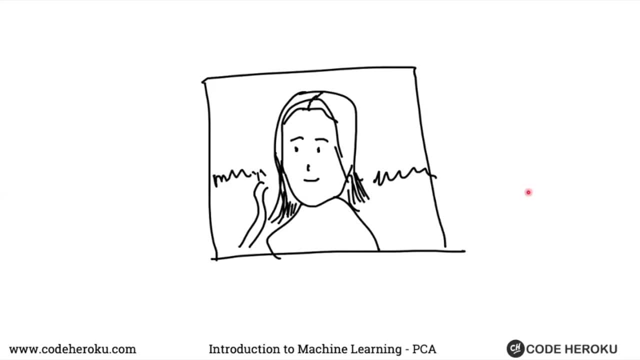 This is as worse as you. You could, You could go. So what are we trying to do over here? We are going to Draw The best version of Mona Lisa, Which is Dimensionality reduction. All right, So If 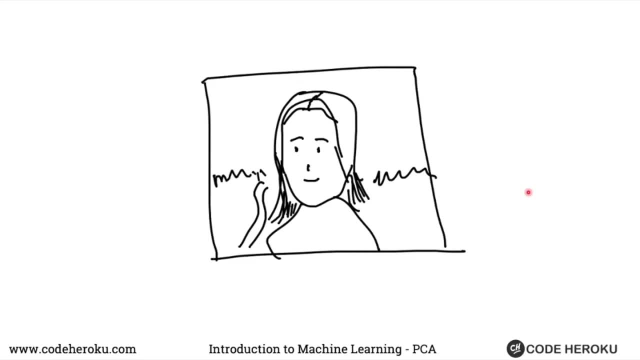 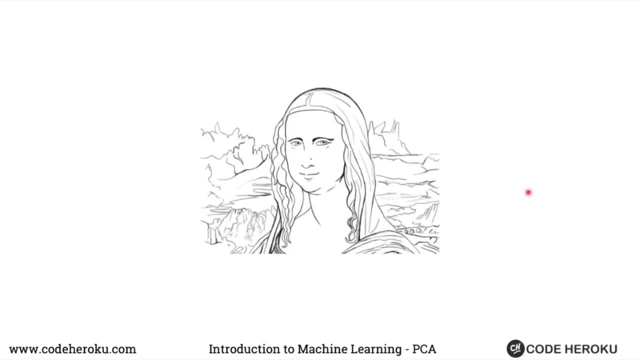 Let's say, You know, Someone was more artistic. They could have also Come up with A better version Like This one. Right, And By looking at this Picture Over here, Will you guys Agree with me? 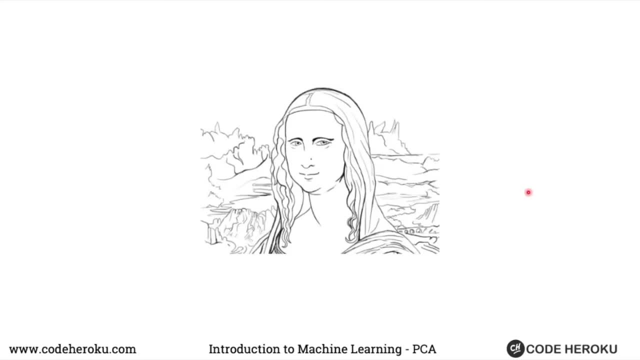 That Just by looking at This image As well Will a person Be able To make out If This is Mona Lisa. A lot of people Will be able To see The painting Of Mona Lisa. 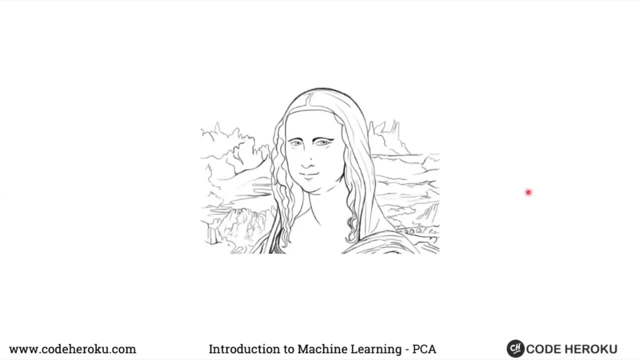 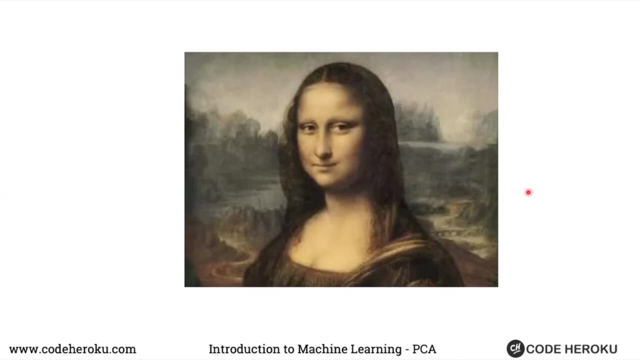 Right. So The point That I'm trying to make Is Over here. This is A much more Higher dimensional View Of This painting. Over here, The image Might be No, This could be. 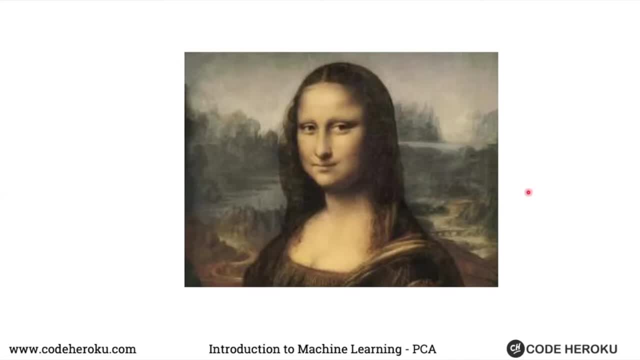 A 256. Cross, 256. Or even more. This is 512. Cross, 512. Pixels, 512. Times 512.. That's A lot Of Dimensions, That's A lot Of. 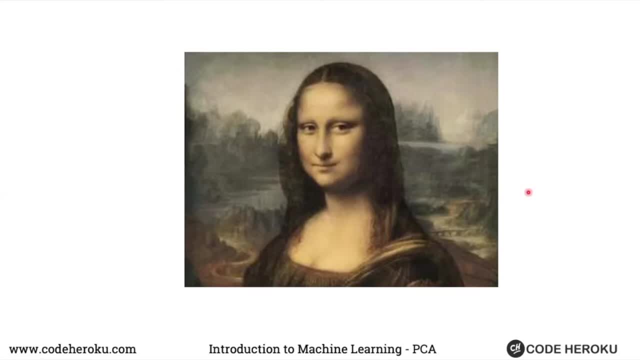 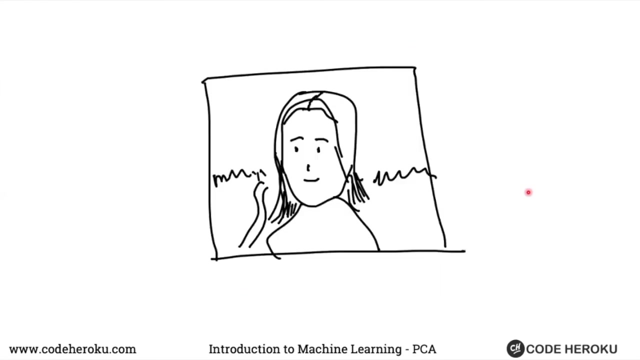 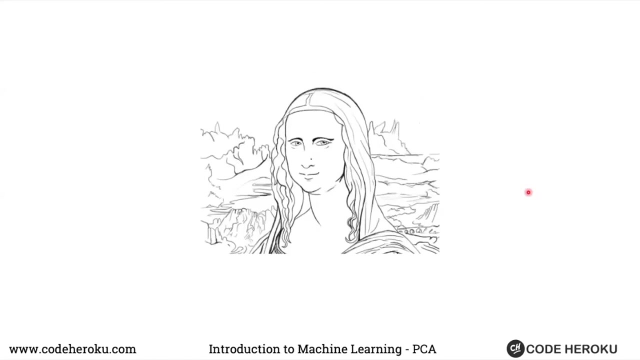 Features. Each Pixel For Our Machine Learning Algorithm Will Be A Feature, But What We Are Saying Is To Our Machine, Which Is Definitely A With. 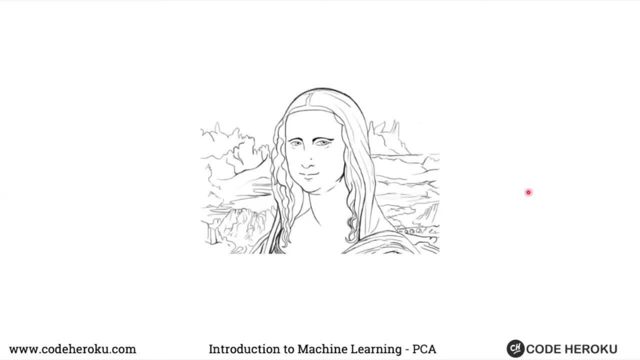 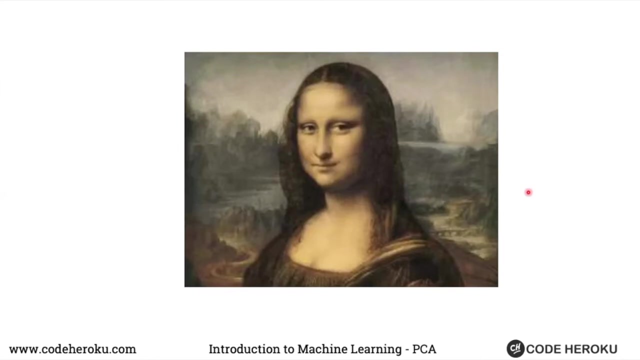 Definitely Needs Less Number Of Pixels, But Still Represents The Same Thing, The Same Underlying Object There. So That Should Give You There Exists A. 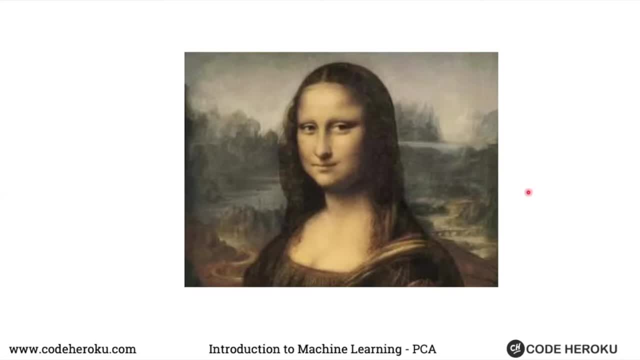 Lower Dimensional Subspace Which Can Still Faithfully Represent Your Object. Does Everyone Agree To Me With That? Over Here We Are Seeing That, Mona. 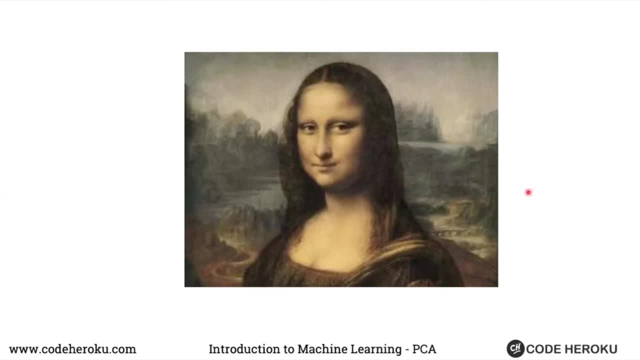 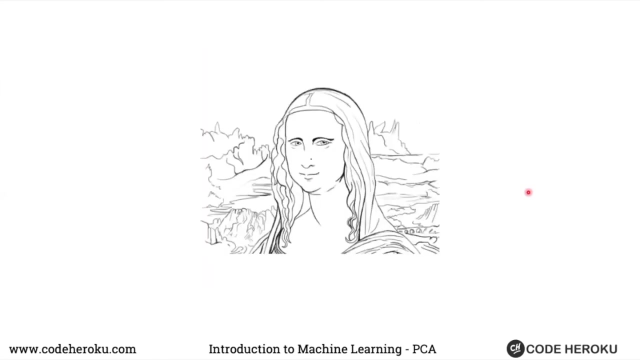 Lisa Has To Make Out From That Image What That Is. Yes, You Could, And Even If, Let's Say, If The Size Was Not Less. 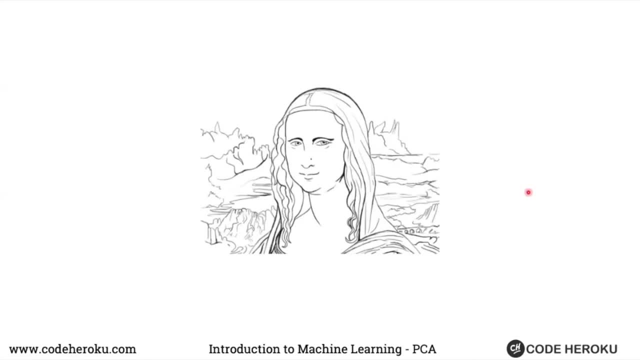 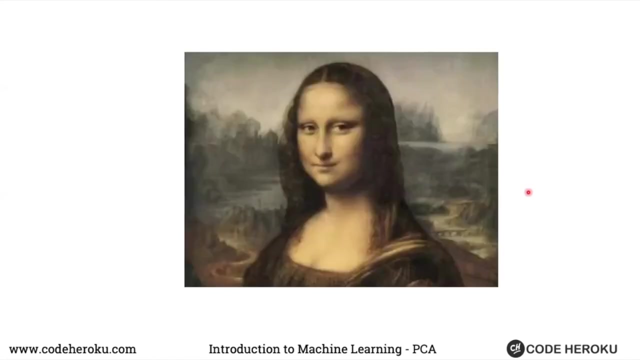 If I Drew An Outline Like Space From What You Already Have In Most Cases, Know It If You Have, If You Already Have Very Few. 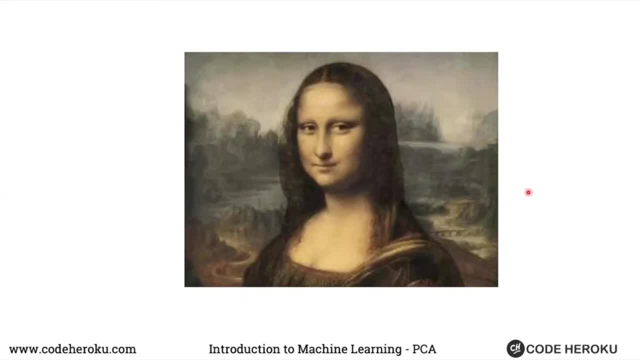 Features. Let's Say, If You Already Have Like Five, You Are Seeing, And That Structure Is What We Are Interested In Today. We Are Interested. 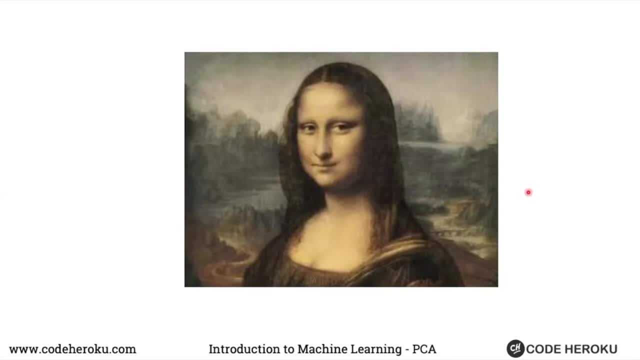 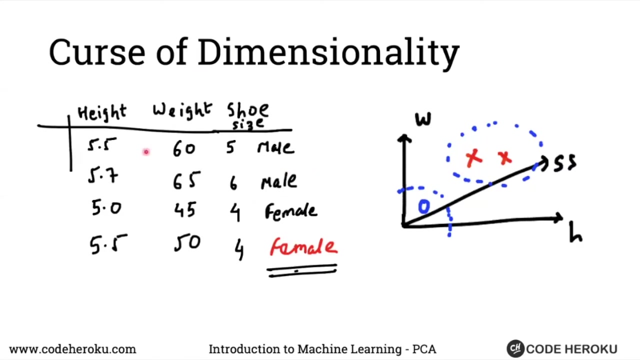 In Seeing. Is There A Structure Or Is There A Pattern? That Might Not Okay. So That's What We Are Going To Try To Do. 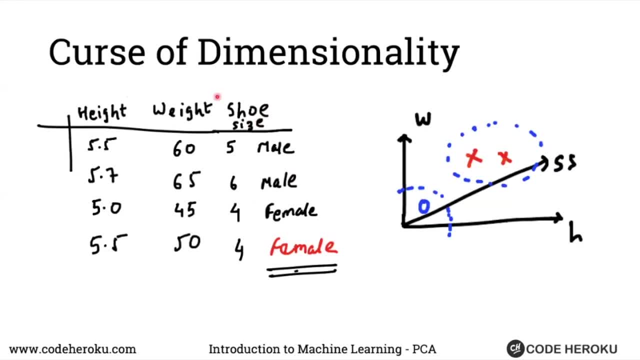 Today We Are Going To Try To Get This Inherent Structure A Lot Of Times. What You Are Going To Make Your Performance Even Worse. 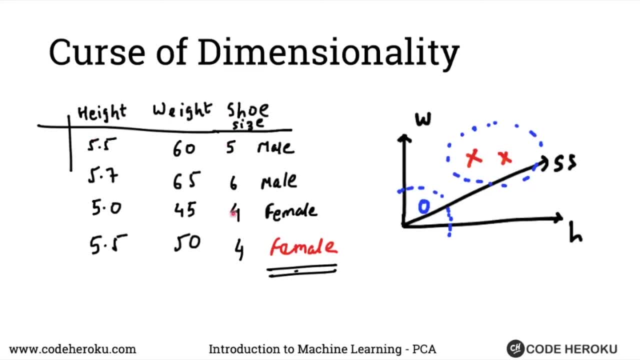 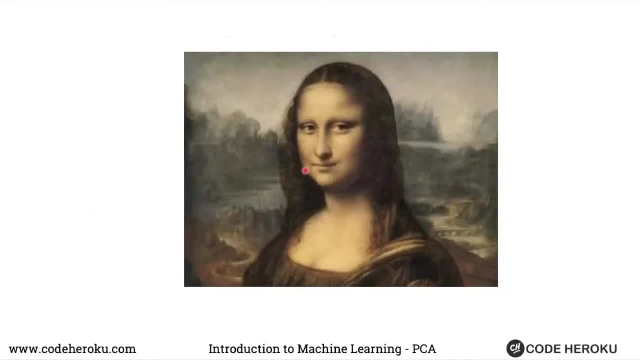 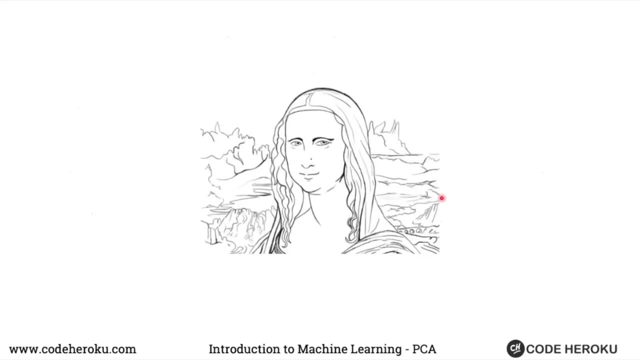 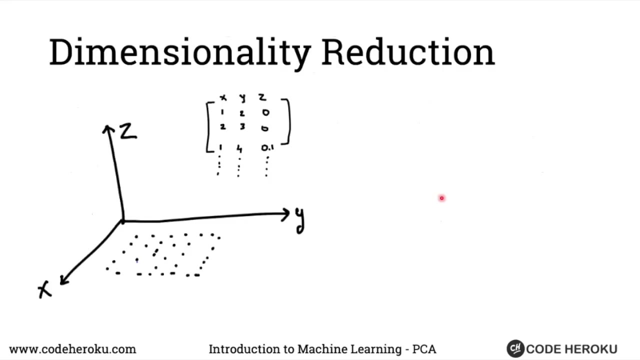 If There Is Significant Correlation Between These Two Variables Or These Two Features Over Here. So When You End Up Having A Z Component Of 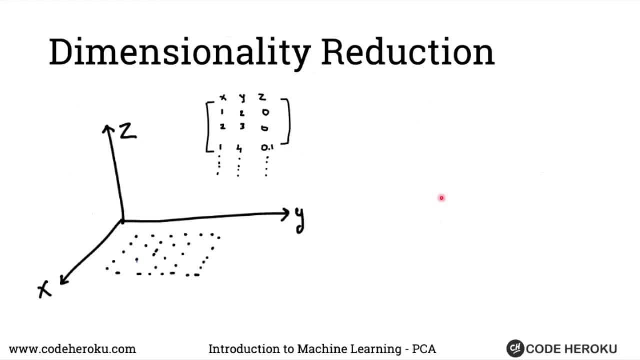 0.1.. But Mostly All These Points Have A Z Component Of 0.1.. But Mostly All These Points Have A Z Component Of 0.1.. 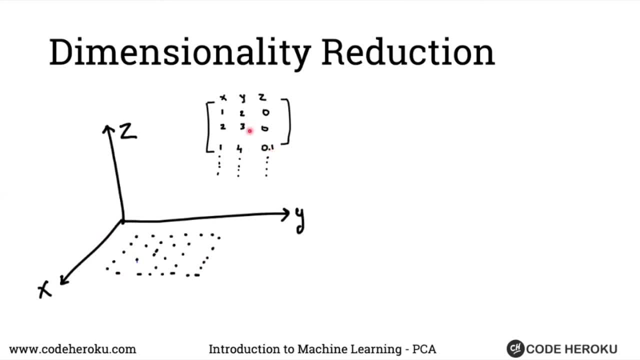 But Mostly All These Points Have Z Component Of 0. So They Are Lying On The Surface Over Here. So If I Were To Tell 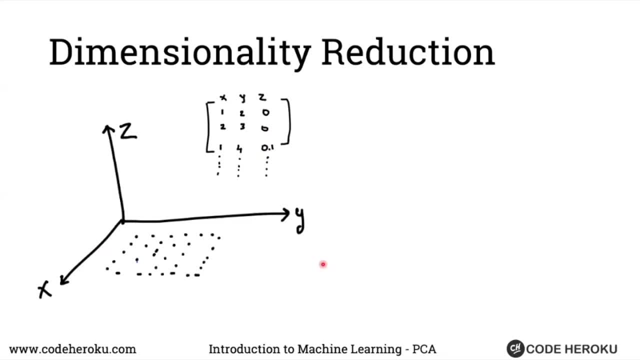 You To Reduce The Number Of Dimensions Is: Even If You Get Rid Of This Z Axis, You Still End Up Representing Your Points More. 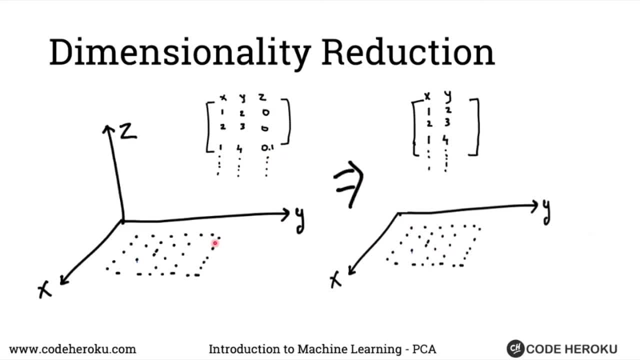 Or Less In The Same Fashion. The Only Difference Might Be The Dimension From Three To One From We Were Able To Reduce Dimensions Going From: 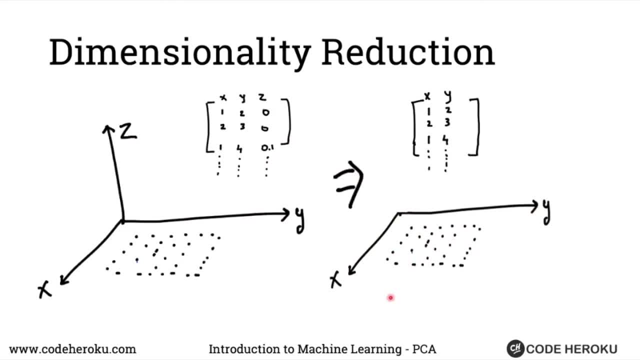 Three Dimensions. We Were Able To Go To Two Dimensions Only Now, Such That Increase- Now I Take Away From This Slide- Should Be We Want. 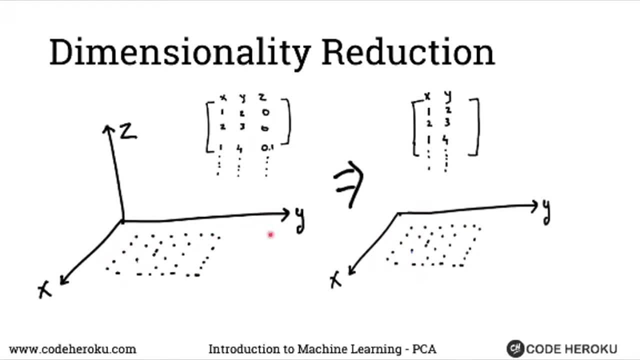 To Preserve The Planes Where We Have Most Variations In Our Data. Our Variations Are Along The Data Like This. Now Have A Look. 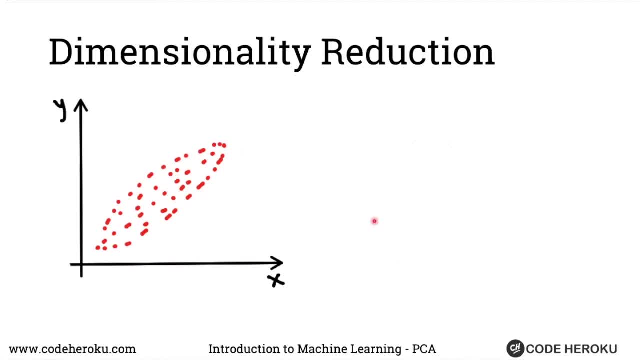 At This Data Over Here And Can You Tell Me If I Want To Go From This Two Dimensions To One Dimensions In Them Right There? 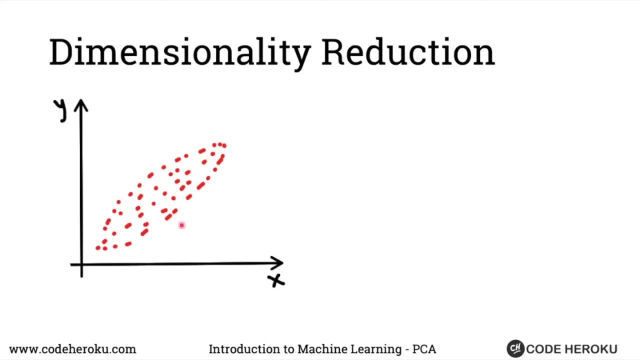 Is Some Variants Along Our Y Direction And There Is Some Variants Along X Direction As Well. So In A Lot Of Cases We Can. 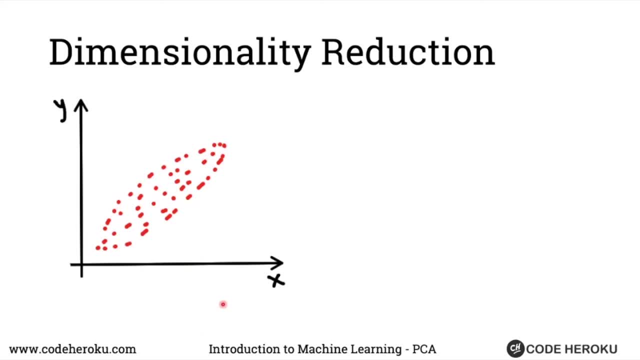 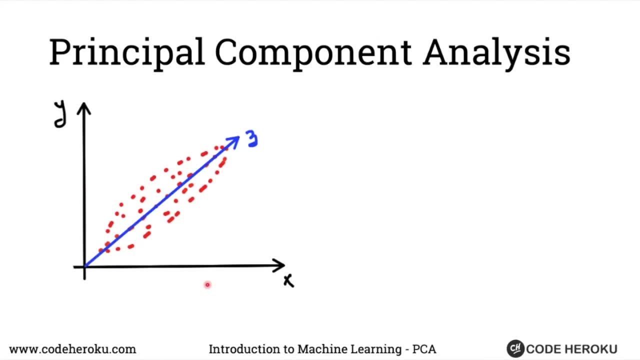 Have A Compact Representation Of Our Data. So What If I Told You, If I Draw A Line Like This Over Here, Let's Say We. 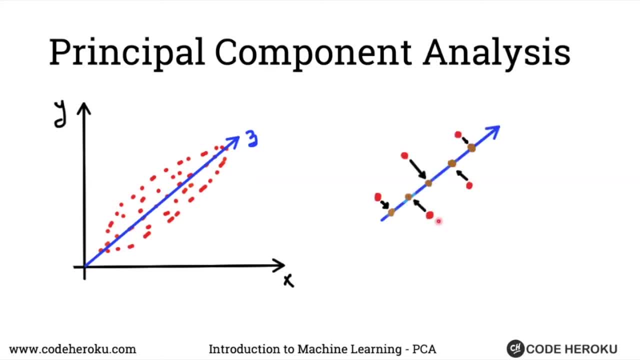 Have A Vector Z Axis Over Here. We Have A Z Axis Over Here And Instead Of Representing Our Data In X And Y Axis, 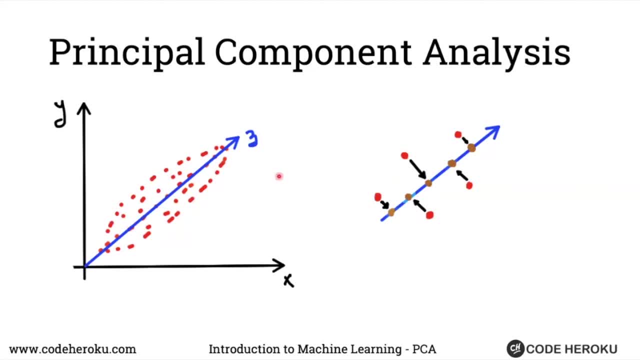 Now What If I Just Represented On The Line- Does Everyone Agree To Me On That, Instead Of Just Dropping X Or Dropping Y? 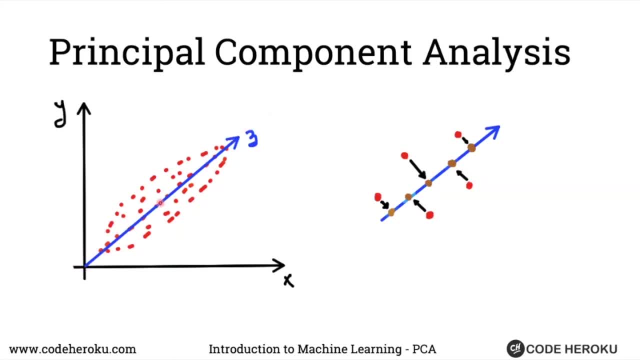 What If We Create A New Dimension For Us? Let's Say Z, Such Projection Is Nothing. But Let's Say: If You Have This Point Over. 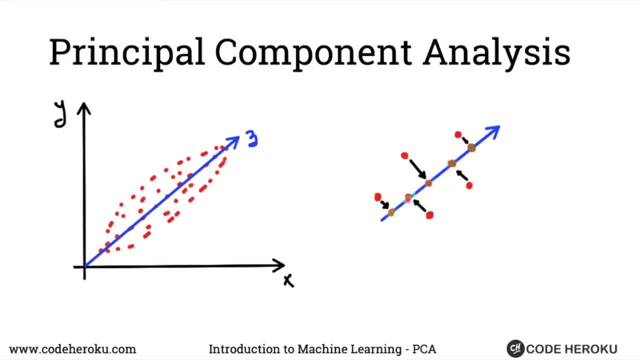 Here You Are Projecting This Point On This Z Axis. You Are Assuming What Happens If It Is In This Data Set, And That's. 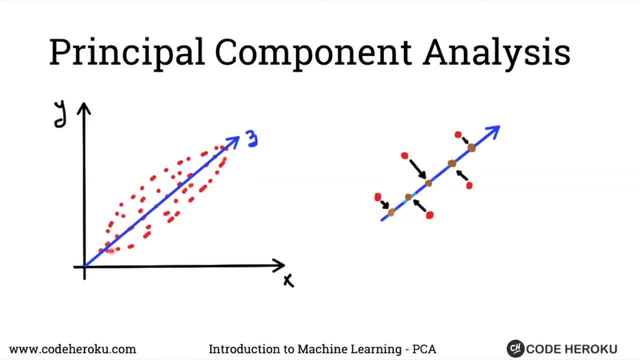 Why We Are. The Name Of Our Class Today Was Analyzing Those Principal Components. Given A Data Set, How Do You Find What Is Still? 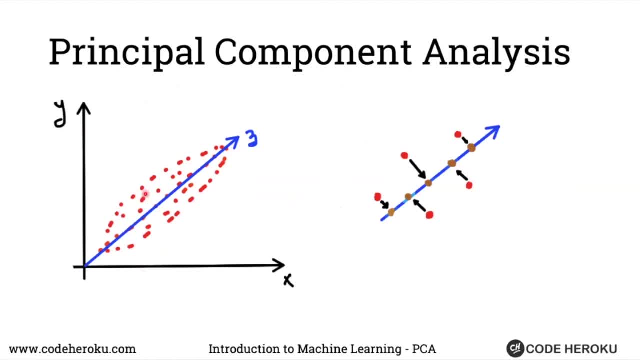 Preserved. Does That Make Sense, So, Intuitively? What We Are Trying To Do Is We Are Trying To Find A Direction Such That These 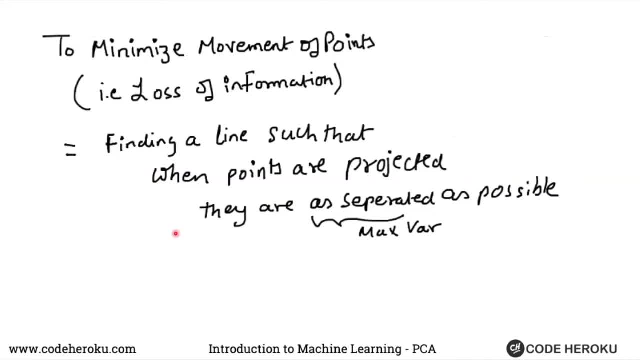 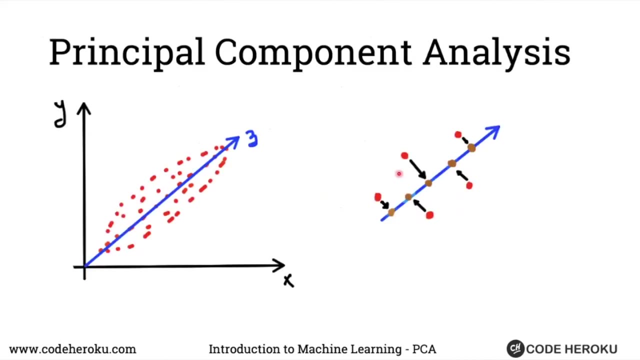 Points Don't Move The Point Of Points, That Is, The Loss Of Information, Is Equal To Finding A Line Such That, When The Points Are, 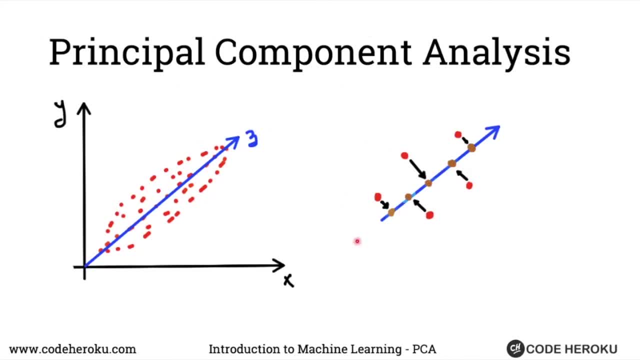 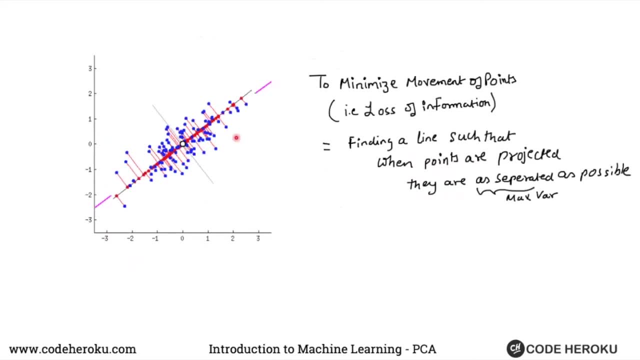 Projected. They Are As Separate As Possible. Now Do You See When I'm Moving This Line? At This Point, This Projection, This Black Line, Is 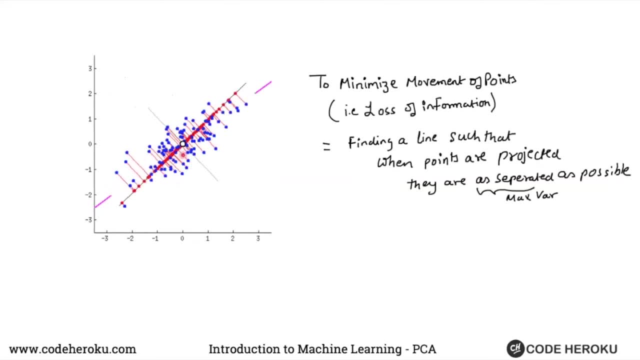 A Terrible One, Because These Points Have To Move A Lot. Now This Is Here, So What We Are Saying Is: If He Want These. 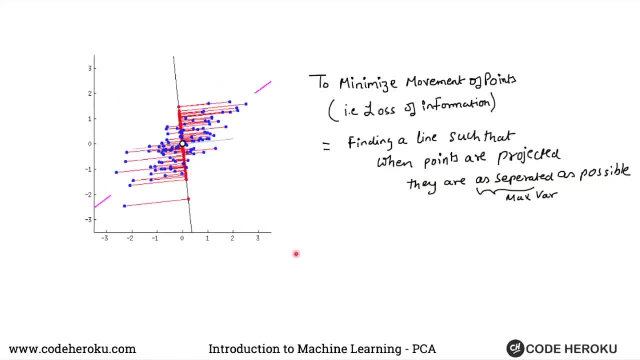 Blue Points And Red Points To Be As Close As Possible. These Red Points Need To Be of a few seconds. let you guys grasp this information that I'm giving that, if you want. 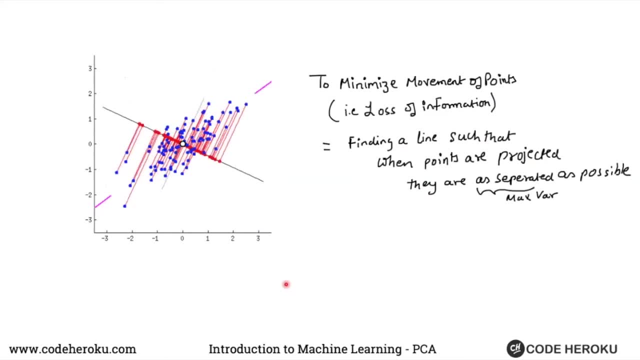 these points to move as little as possible. so we want these, this blue point, to be as close as this red point as possible. that is nothing but is equal to saying that finding a line such that these points are as far apart on the black line. these red points need to be as far apart on the. 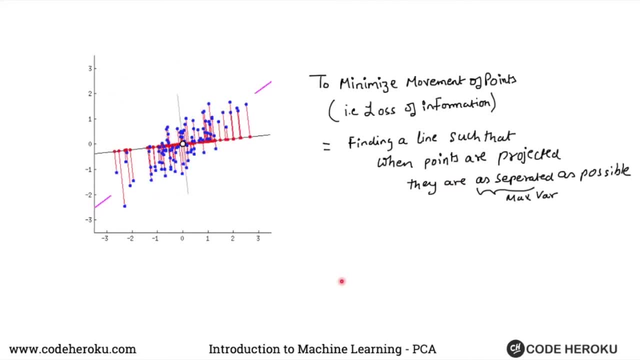 black line as much as we can. we are trying to find a line which will have maximum variance when these points will be projected. okay, so let's try to formalize it a little. so let's say again: I have this plane over here now. we have already told that there exists a direction such that 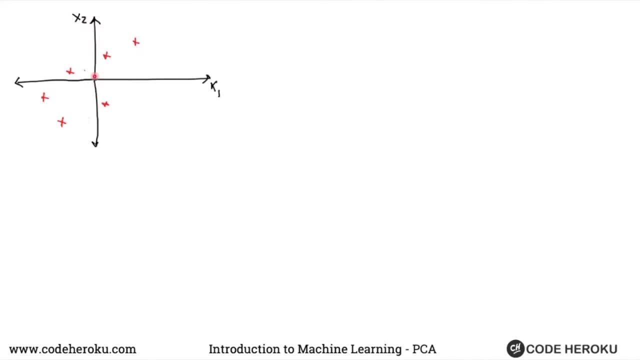 if we use that direction, we want these points to have maximum variance. so over here, just by looking at the graph, we can say that this line over here, something which is going from the origin over here, so this line or this vector will have, will be the line. 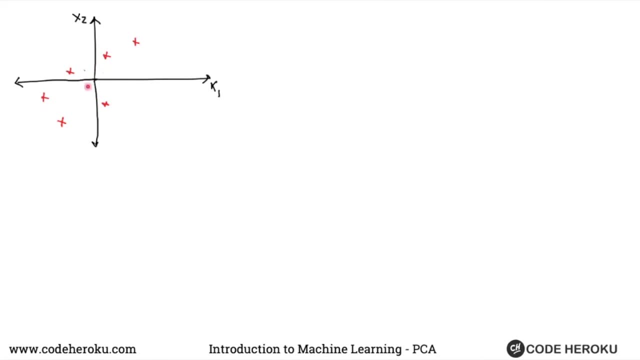 which will have maximum variance. so the maximum variation in this data set, just by looking at it, will be around this line. we have a quantity for us called as covariance of a matrix. so covariance in this data set is given by you. just take each X size and multiply that with the 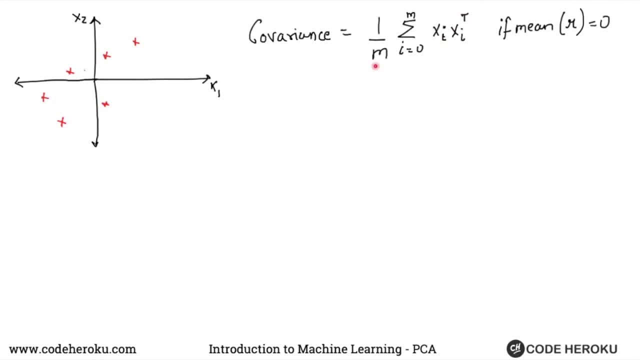 transpose of X, I and you average it out so that will give you the covariance if the mean is 0 and we have the mean as 0. over here is all these points. we are assuming that they are centered around origin. so we are. we know that the covariance of this data set is going to be. 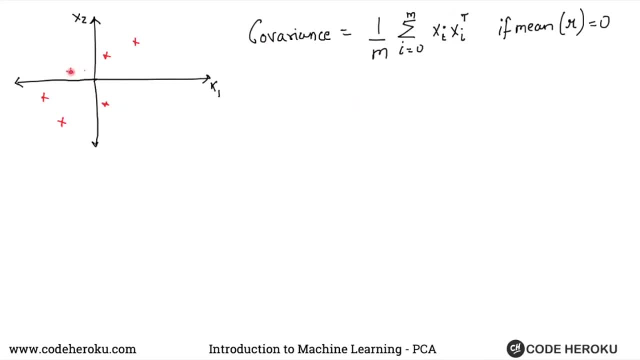 here. so in today's example we are assuming that the invariance of this data set over here is given by each point multiplied by now. you, you take all excise and you multiply by a transpose of X, I. that will give you the covariance. and let me also tell you that covariance in this, if you, 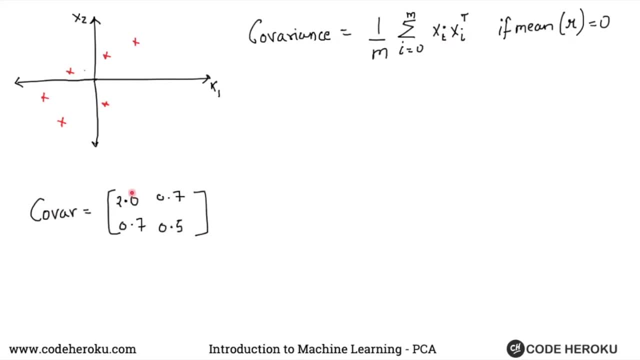 do this math over here for this data set. let's say, this covariance is no matrix that you get. now I want to show you, instead of deriving PCA, I want to show you what happens, an interesting observation that we have. so let's say, if I multiply this: 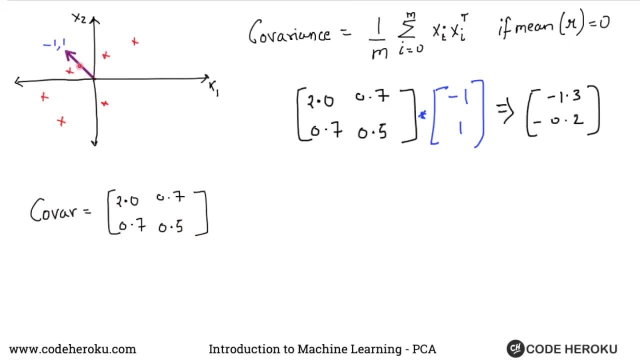 Let's say, if I multiply this, the value of X equals 30.. multiply, take any random vector over here. so I took a vector minus 1 comma 1. and what happens? if I multiply this with the covariance matrix, I get it's something like 1.3 minus 0.2. okay, so if you multiply this covariance matrix with 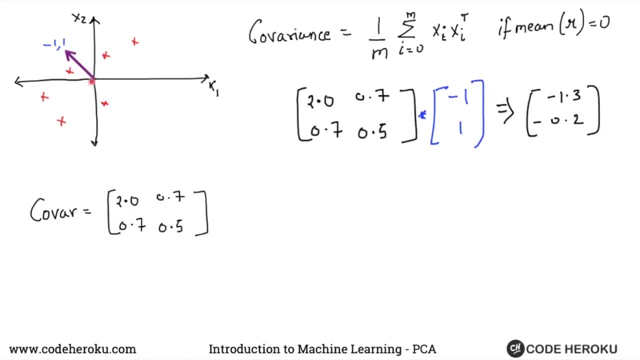 any random vector. so let's say I took minus 1 comma 1. that will give me minus 1.3, minus 1- 2. so this minus 0.3- 0.2. if you plot it on the graph it will be somewhere over here. so minus on x-axis and minus negative on the y-axis as well. 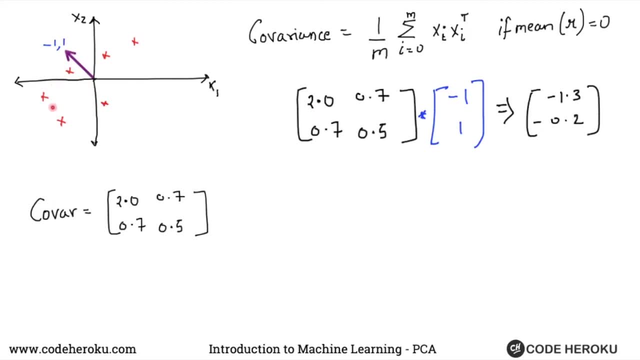 so it will be in this quadrant over here. so let me just put it over there. so we got this new vector. what happens if you multiply it again? what you get is minus 2.74, minus 0.1. so again we are in the same direction. we are in the same quadrant over here. 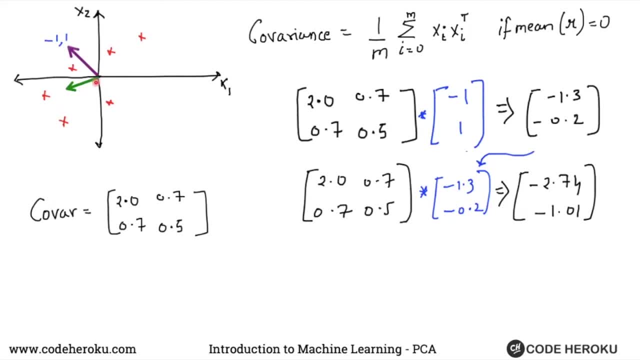 but our vector, which was initially it was minus 0.13 or minus 1.3, now it is minus 2. so our vector is getting bigger but it is rotating less. so now we are somewhere over here in the blue and if you multiply it once more, what you will? 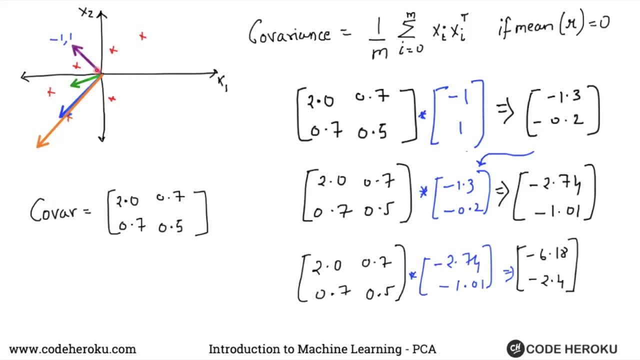 end up seeing is this vector is getting rotated in a direction of the maximum variance. eventually, even if you keep on multiplying, as you see it is, we are converging to something over here. initially our rotation was quite large, but ultimately what happened is we kept on decreasing the rotation, but our length of vectors keep kept on increasing. 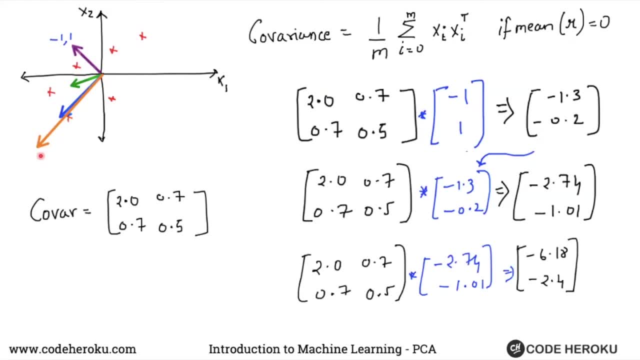 so I'm trying to show you an interesting observation about the covariance matrix. and why are we dealing with covariance matrix? because we are interested in maximizing the variance. and what we are seeing over here is if you are given a covariance matrix, you multiply that with any random vector. in this case we are taking minus 1,1. that vector will get 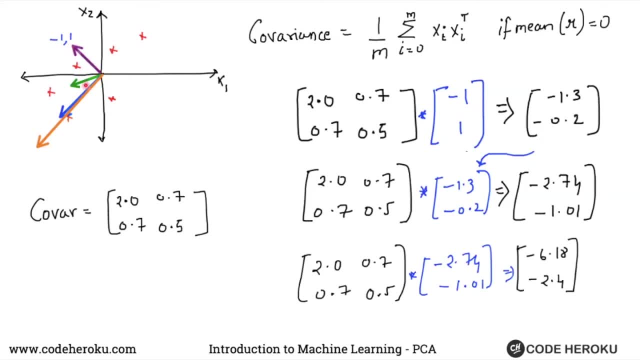 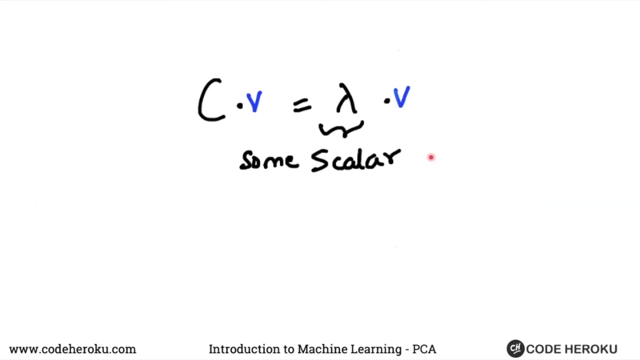 rotated by a certain degree and eventually it will stop rotating lot more. it will converge to a point which has the maximum variance And in this case we converge to this orange vector over here. and this problem seems to be familiar to you, right, if you have taken mathematics in your engineering classes, or 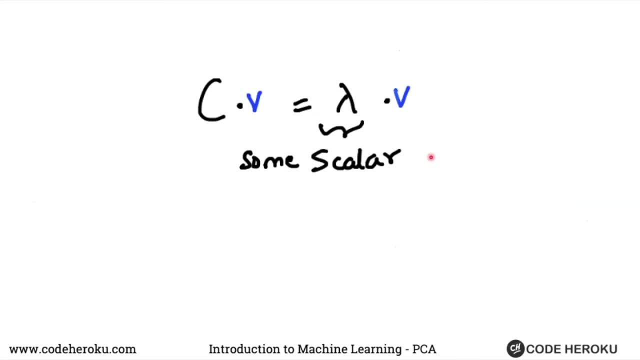 know if you have taken advanced courses with matrices. has anyone seen something like this before? Yep, Rakshita got it right. Egan vectors, Right, Okay. So what we are essentially saying is: coming up with this is nothing but doing an Egan. 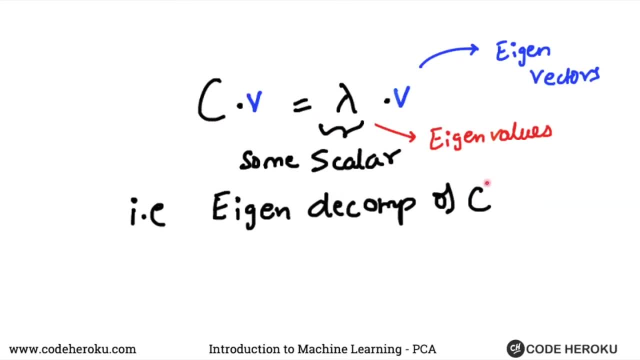 decomposition of this covariance matrix C. It happens to be that these lambdas are also Egan values of this covariance matrix and the vector V itself are the Egan vectors. Now let me give you some properties about these Egan vectors. The vector V times V- transpose- is an identity matrix. 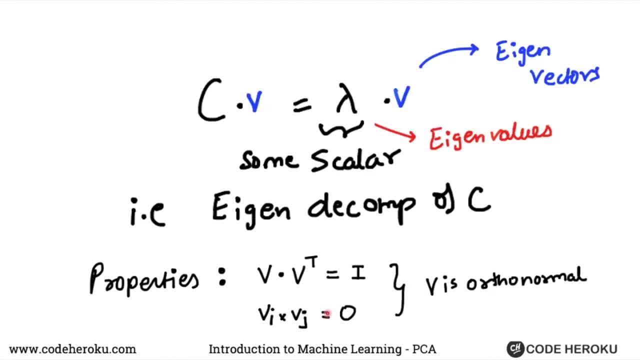 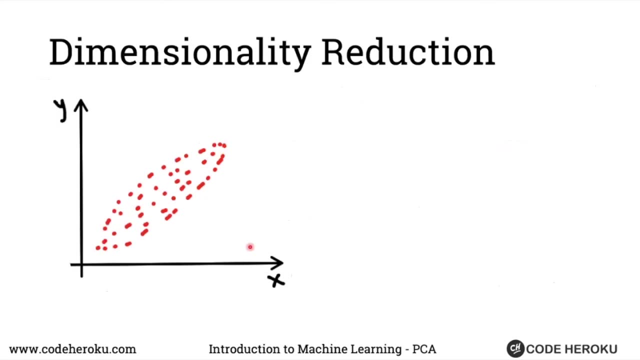 We don't want any correlations or these vectors. The first vector and the second vector are going to be orthogonal to each other. Okay, So we have already seen that. why do we need that? right, because over here we said that if the shoe size was dependent on height, 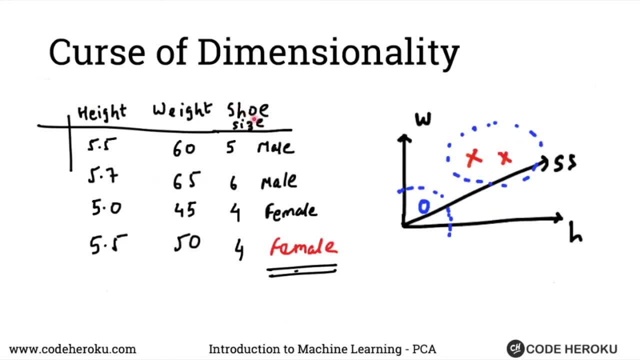 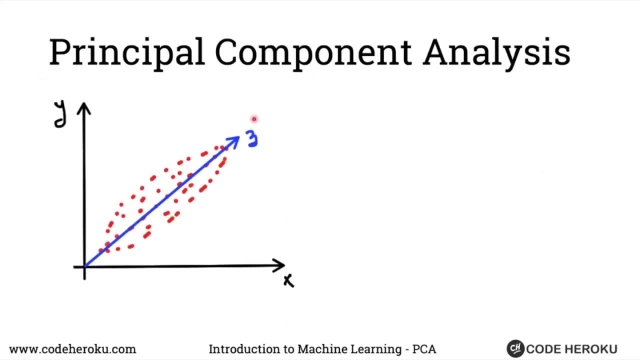 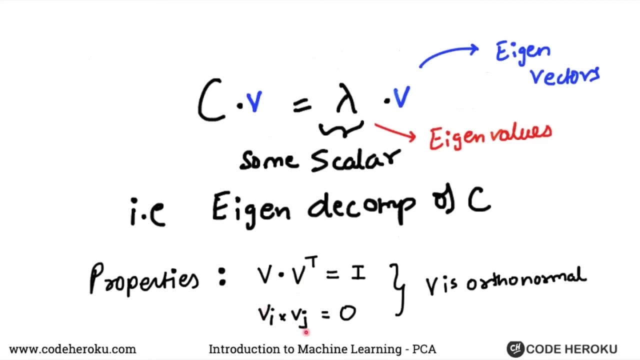 We want to get rid of this shoe size. Okay, So that's what, intuitively, PCA is trying to do as well. It is trying to find directions which are orthogonal to each other. So we are: VI times P- transpose is identity matrix, and VI times VJ is zero. 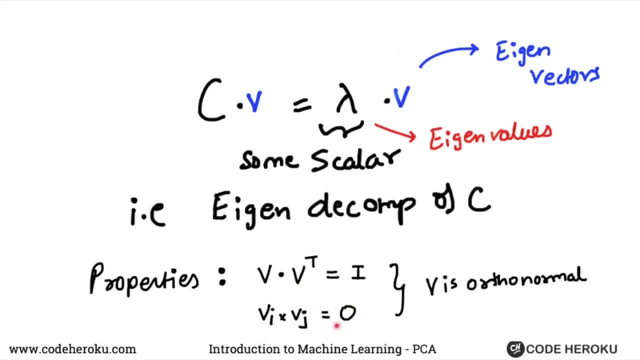 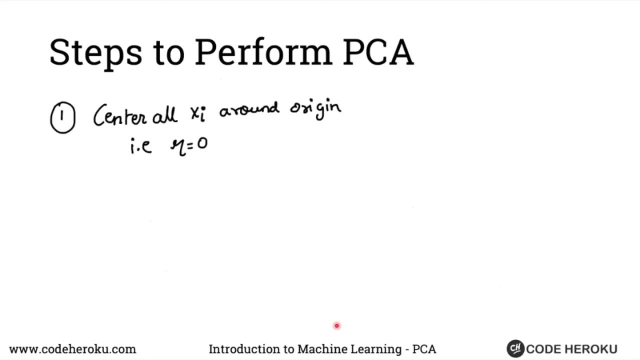 There is no correlation between the two components of that vector. Okay, So here are the steps to perform the PCA. What we will do is First center all our Xi's around origin, so that our math becomes much easier down the ground. So we will center all our data points around origin. 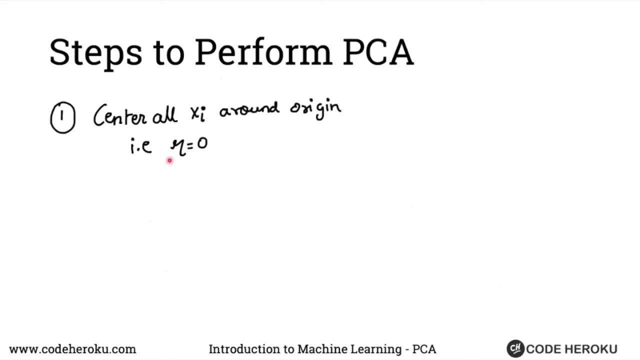 So we need to scale all our data points so that their mean is zero. Second step to do: PCA, as we saw, will calculate the covariance matrix, and this covariance matrix is nothing, but you take Xi and you multiply it by the transpose of Xi. Okay, 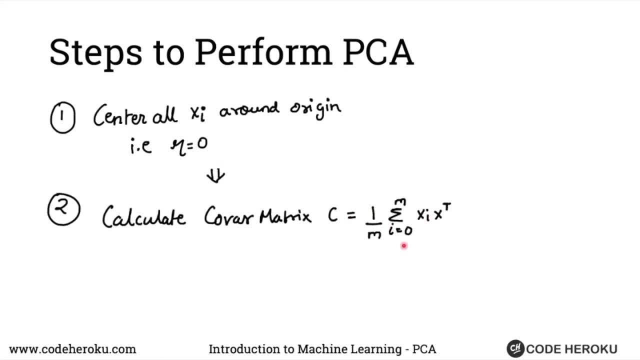 You average it for all by divided by the number of points that you have. This will give you the covariance matrix. and third, we already saw was: given this covariance matrix, We want to calculate the Egan vectors and the Egan values of C, so that the Egan vectors 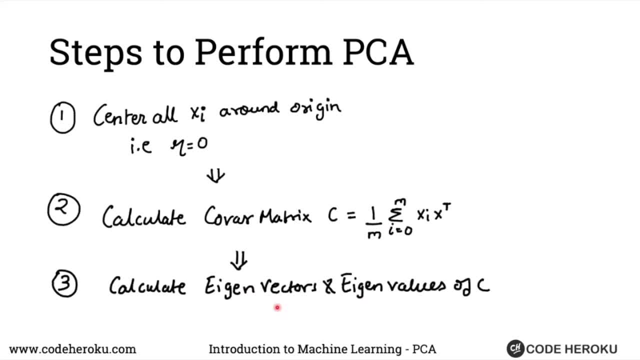 will give us the direction where we have the maximum variance. What we do is we take all these Egan vectors and arrange them Okay In a matrix like this one, and we arrange them with increasing order of their Egan values. So if Lambda one was the Egan value corresponding to V1 will have this as first, then V2, V3 and 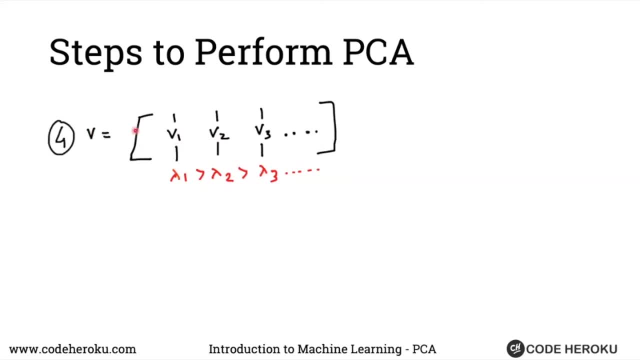 so on. So we create this matrix V such that this Egan vectors are in ascending order or descending order of their corresponding Egan. Okay, This is the Egan values. Then what we will do is: the whole point of this exercise was to reduce dimensions, right? 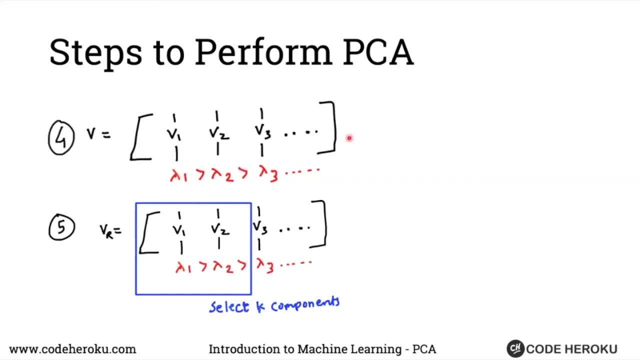 over here. This will be an M by M matrix where, if M, if we have M dimensions, there will be an M square matrix, which is too high. We don't want that. We don't want those many dimensions. What we could do is actually take just a subset of all the vectors that we have. 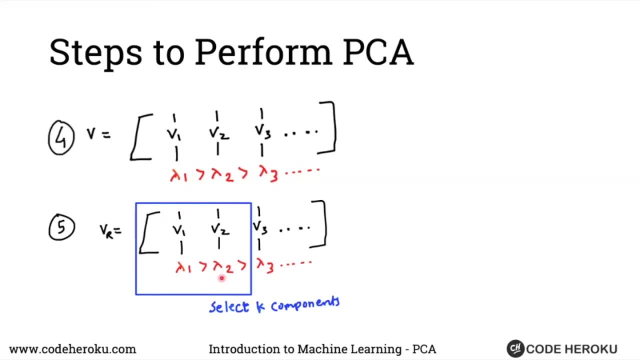 Okay, And the reason why we could do this is this: Egan values, which these vectors correspond to. they tell us, they give us a sense of how much variation that Egan vector captures. So, over here, the amount of variation that your reduced subset will retain will be given. 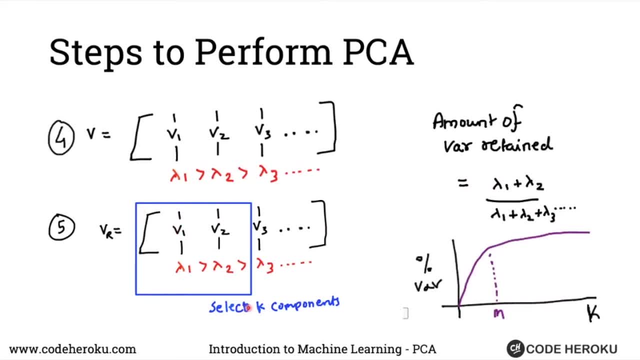 by Okay. So let's say we are just taking two vectors over here, Okay, Corresponding to Lambda 1 and Lambda 2. the amount of variations, or the amount of variations that we are retaining, is given by Lambda 1 plus Lambda 2, divided by all the Lambdas. 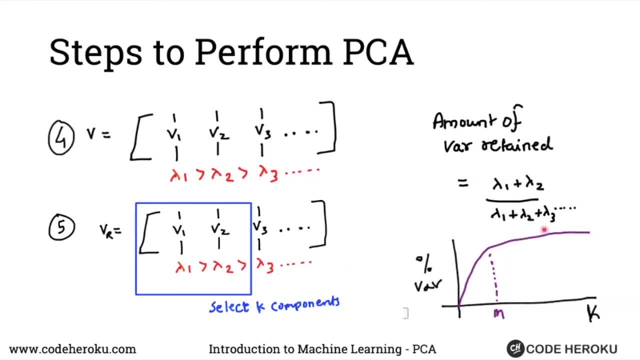 Okay, So this will be. this will give us amount of variation that we are retaining in this data. So if you plot a chart, it could be something like this one over here: you have K, number of components. You have principal component one, Two, three and so on. 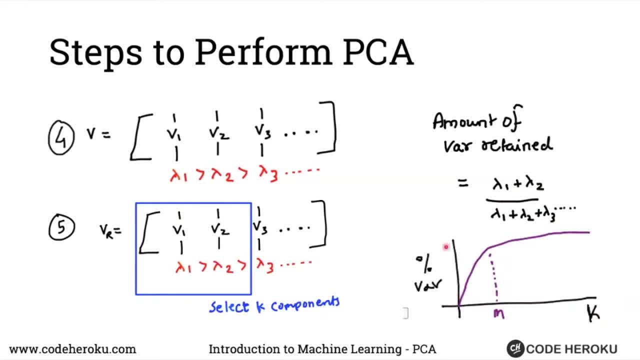 And you will see a graph like this. So the percentage of variation that I'm capturing in first few Egan values will be lot higher after a point. it just know we are just getting incrementally better increase in the variance. initially first few components, it will increase exponentially. 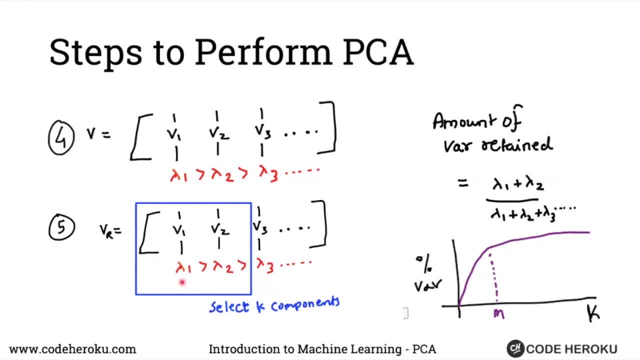 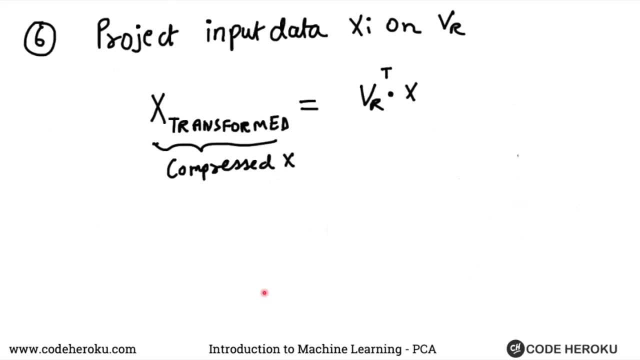 So that's the reason I can just take two components and still get a better or a close enough representation Of my data. Next thing that we want to do is we want to project this input data that we have. The whole point was to get a compressed representation of our data points. 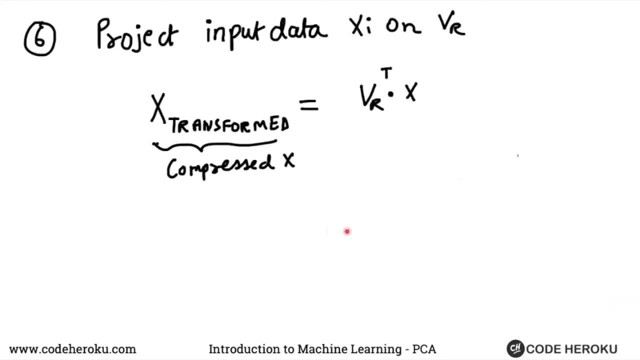 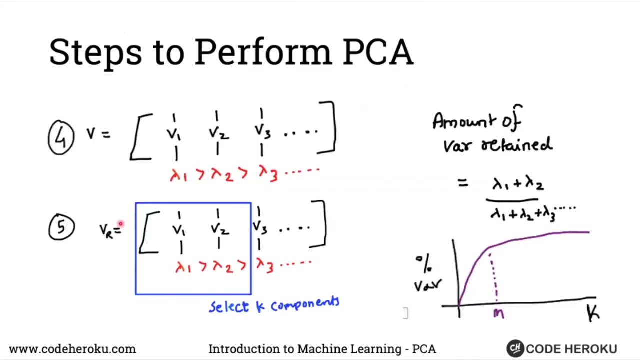 Right. So the whole point was to project our data set on to something else so that we can get a compressed representation. So what we will do is we'll create this new Vector, X transform, Which is also the compression representation, Okay, representation of x, such that we take this vr, this reduced subs, vector, subspace that we got. 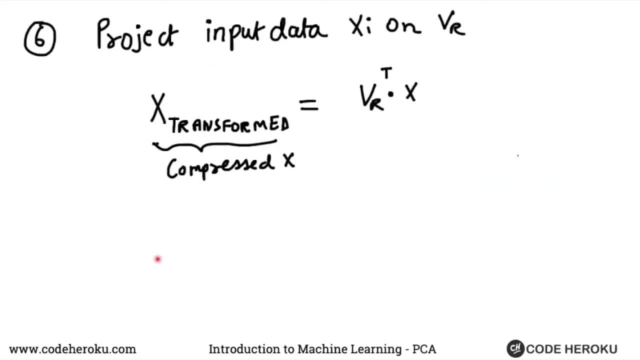 over here. so this is the vr and we just transpose it and now apply to x. so this is nothing but projection of this points on to vector vr. okay, so we got this x transformed, or this is the pca representation in pca subspace or in the pca world. we are saying that this xi in pca form is nothing. 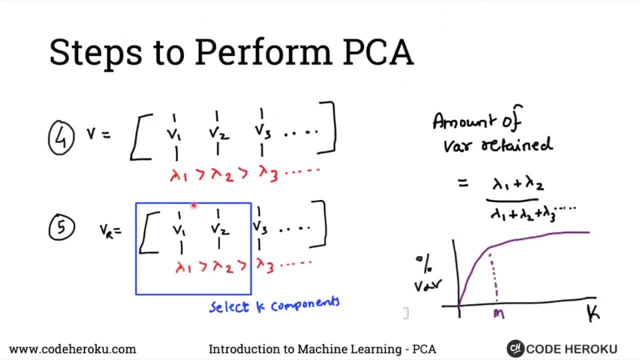 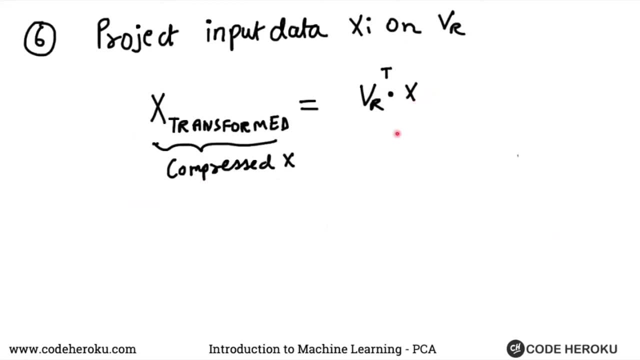 but this vr matrix that we got from here, transpose it and multiply that with each x. okay, okay, okay, simple. let's say, if you have to recover this information, let's say, if you have to go back from x transformed to x again, how do you, how would you do that? if you take, multiply both? 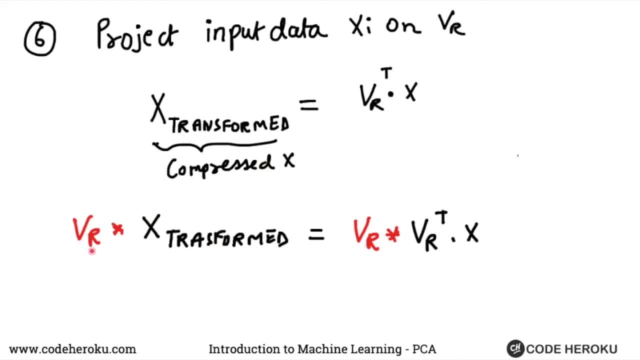 sides of this equation over here with vr, what will? what you will end up seeing is this: vr times vr. transpose is a unit matrix, because that's a property of our egan vector, because, because this is one, this will be equal to x itself. right, so this part will become one. we still have x. 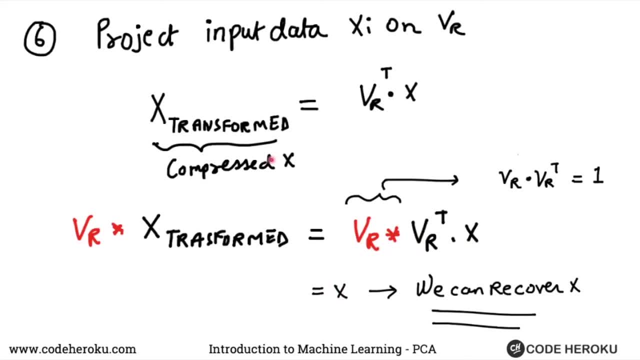 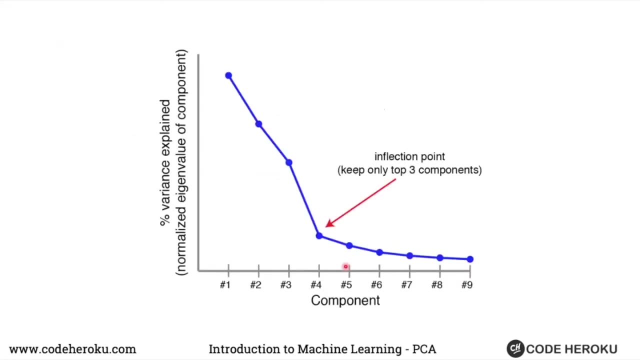 so what we are saying is: even with this transform space, if you multiply the transformed version of your vector with vr itself, you will end up having the original x, that is, we can recover x. this slide is just another version, another way to represent this graph over here, and so sometimes you 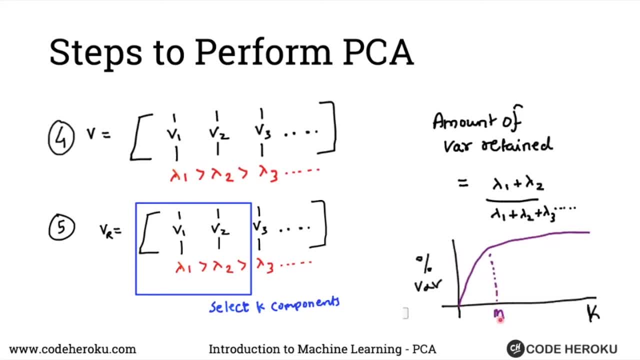 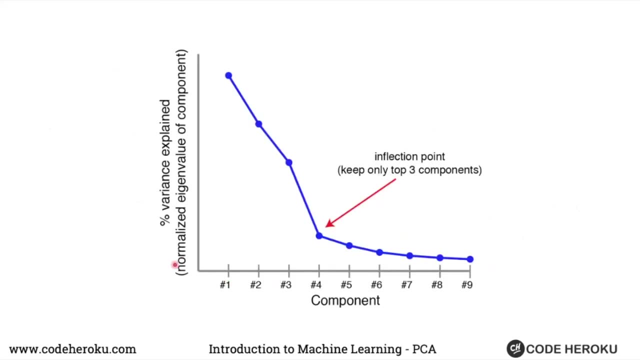 see people you know selecting m or how many principal components to keep, by looking at this chart, which is a cumulative sum of all the variation which is retained and over here. you could also, or another way to put it is now, by looking at this chart over here. so with each for the first, 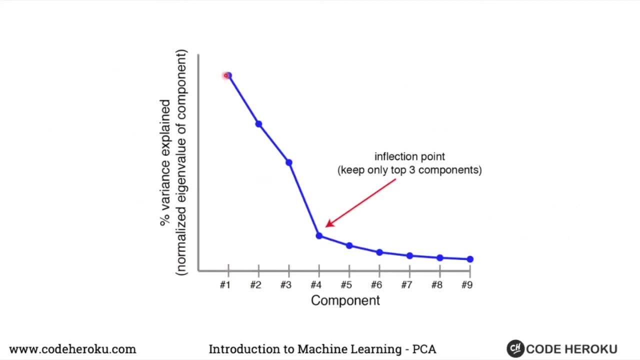 principal component, you will have maximum variation, which is getting captured from. second, you will capture a little less. in the third principal component, you will have even less and after a point now you will stop reducing. so this is very similar to the the elbow chart that we saw for knn. right at this point we say, okay, it doesn't help anymore. 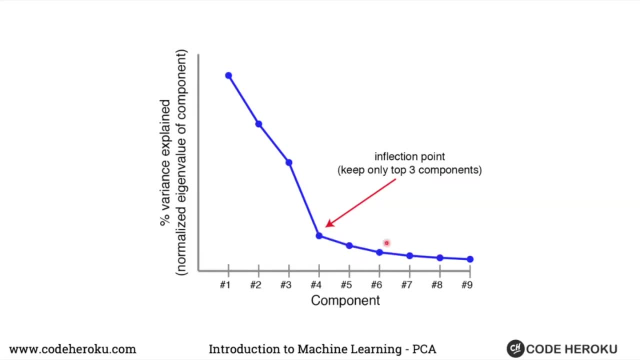 after this point, we are not capturing enough variation in our data, so we can, in this case we can- select principal components for number of principal components, or we can just keep top three components in our data, so we can, in this case we can, select principal components for number of. 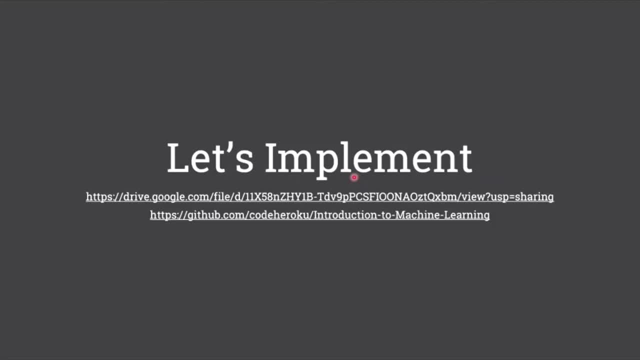 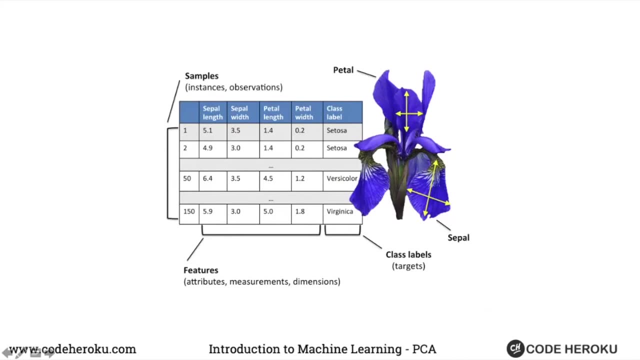 over here. so let's go ahead and implement pca. what we have in this data set are four features of this flower. so what species of this flower it is? so, is it the setosa or the other? the rest three of these? okay, so these are the features and these are the labels. this is the data center we are. 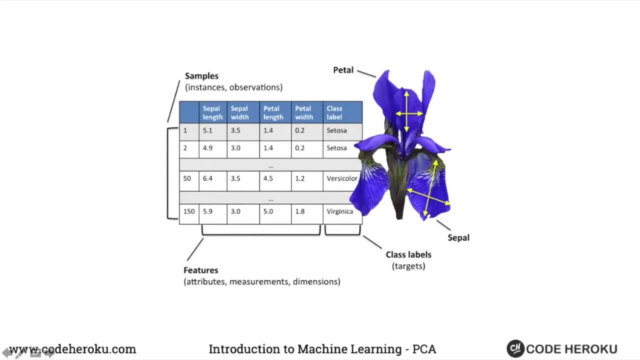 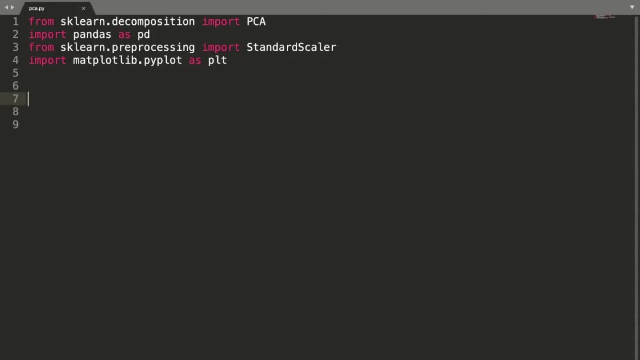 going to work on today. we are going to try to see, instead of representing in this four feature space, is there a better representation that we can get in pca subspace? so what we are going to do is as we do usually: we are going to load our data set using pandas library. so go ahead and do that. so 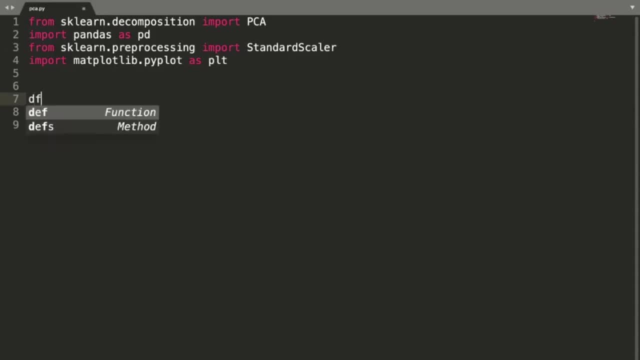 what we are going to say is: data frame is equal to pd dot- read underscore csv. pd dot- read underscore csv. and guys, we have done this several times in our previous classes, so i'm just going ahead with this. so i'm going to say iris dot- csv. 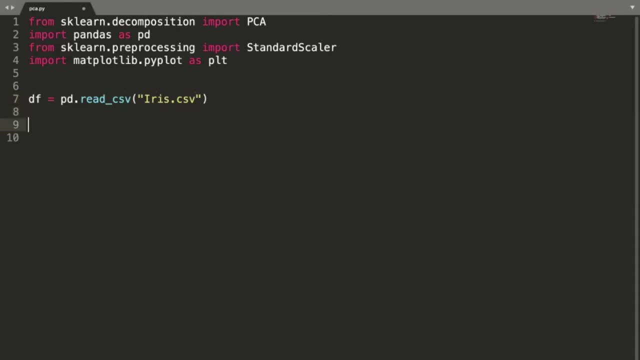 now what we need to do is: let's look at the data frame and let's see what do we have over here. so let's say, print data frame so that we just print out the first few rows over there. okay, so we printed the first few rows over here. what we see is these are our. 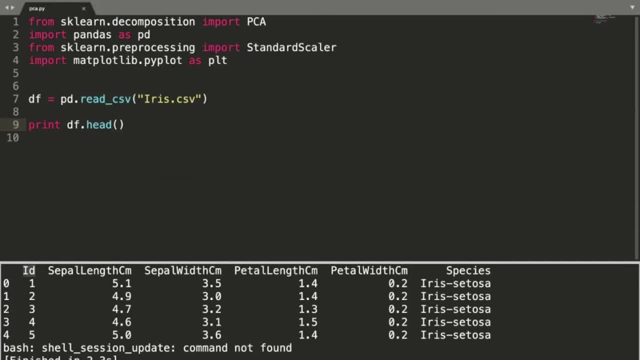 the first few rows over here. what we see is these are our columns in our data frame. we have an id, we have sepal length in centimeters, the width, the petal length and the petal width, and this is the species, which is the eventual classification label, if you. 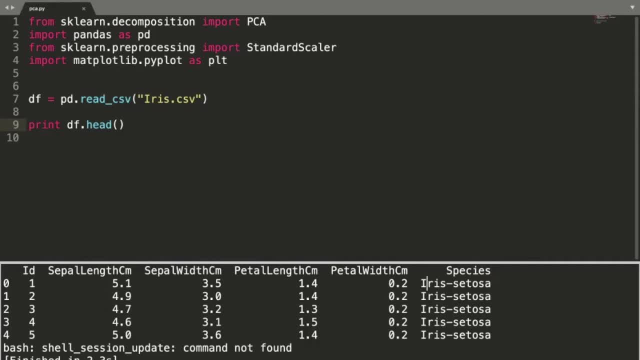 do a classification. if this is for a classification, this is what you would use for your labels, right? so let's go ahead and take the features. let's separate out our features. so what we need to do is let's just say: let's take labels over here first. so i'm going to say labels is equal to now. this can be after this. 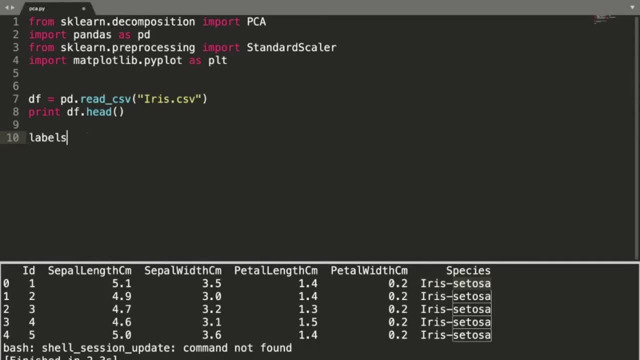 so we need to say labels is equal to data frame of species. right, i'm going to say species over here and then i'm going to say x, i'm going to make all my. take all my features together. so from data frame i want all my features, i just want the features. 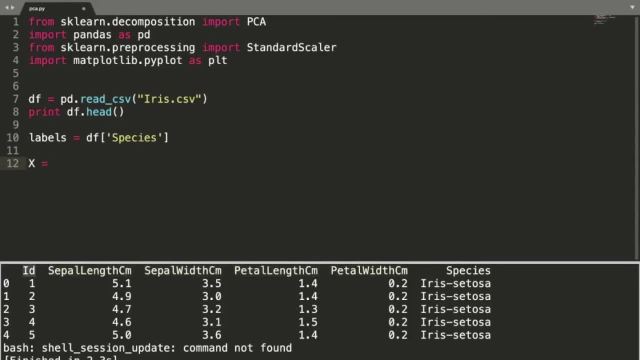 i want all my features, i just want the features. so what i could do is just drop the id and the. so what i could do is just drop the id and the species over here, right? so x is equal to data species over here, right? so x is equal to data frame of need to drop. you could say id. 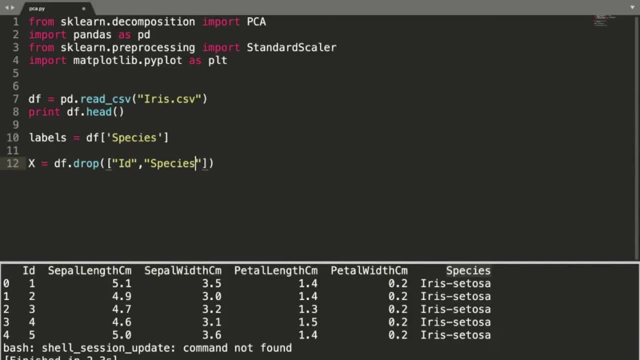 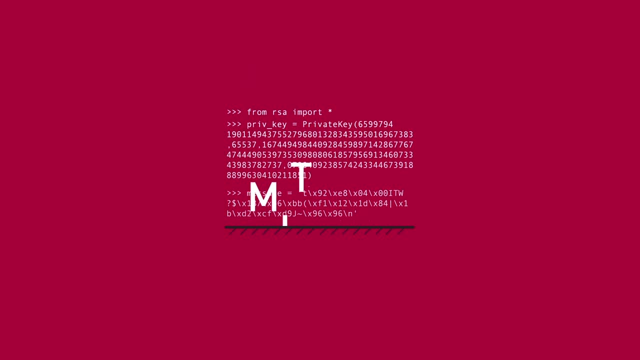 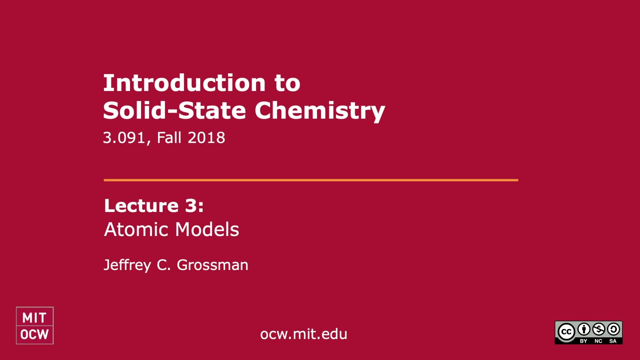 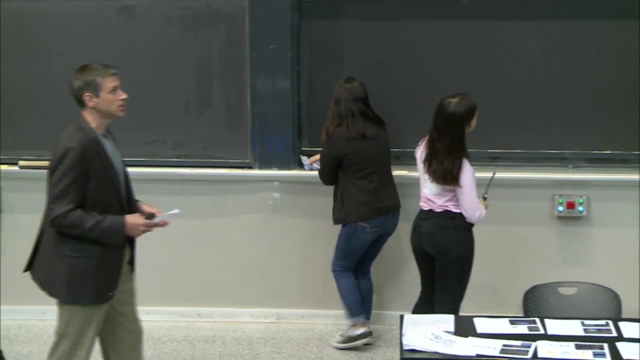 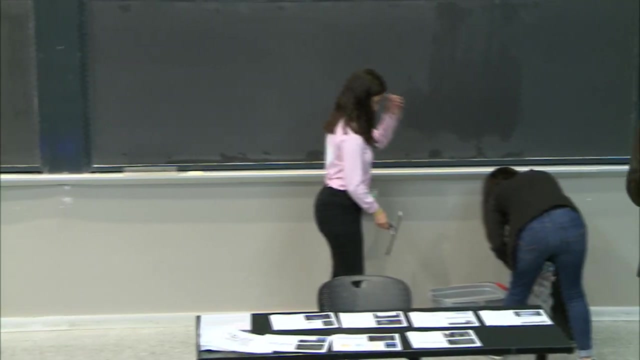 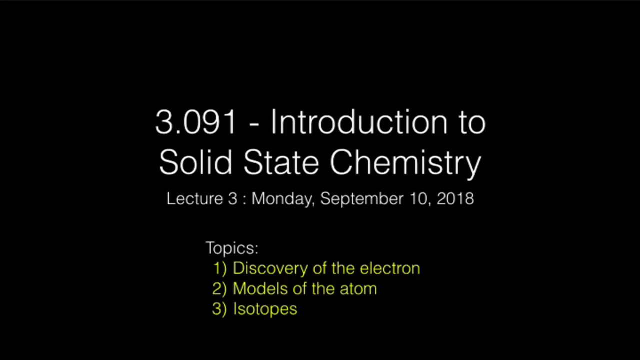 Welcome to the third lecture of 309.1.. Let's get started. Today is a very exciting day because we are going to discover the electron together. That's our goal today. It's right there: discovery of the electron, And we're going to start talking about models of the. 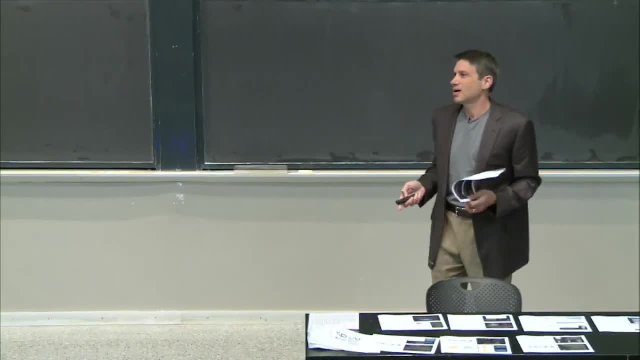 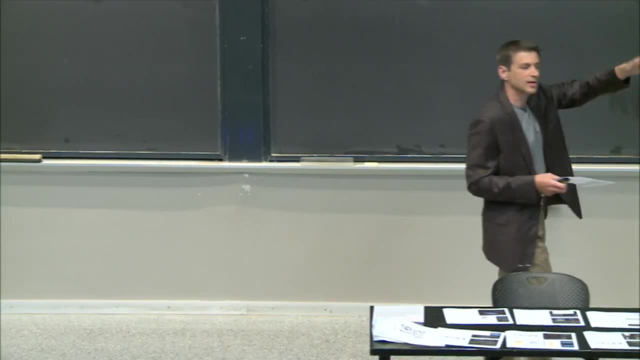 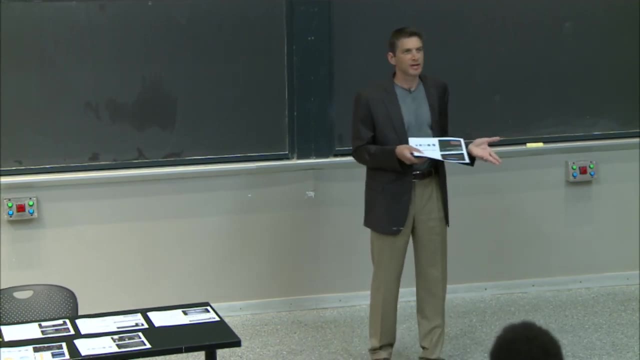 atom. Before we do that, I want to count. I want to count because that's what we did on Friday And we'll use this problem actually twice today, By the way, like if I do a problem in class and it's like in a goodie bag and stuff. I don't know, it might be the kind.